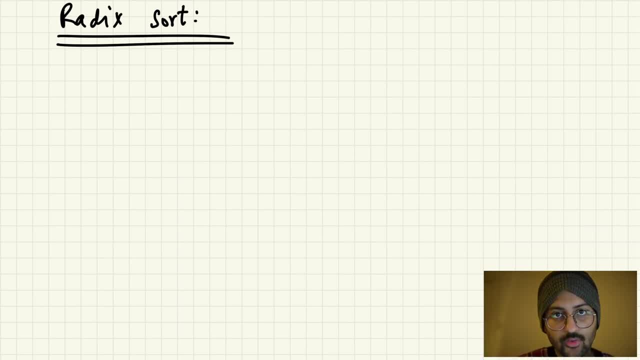 we'll see what is radix sort, what are the advantages, when to use it disadvantages: the theory, the implementation, the dry run, the code itself. So let's get started. So let's see what radix sort is and how it works. 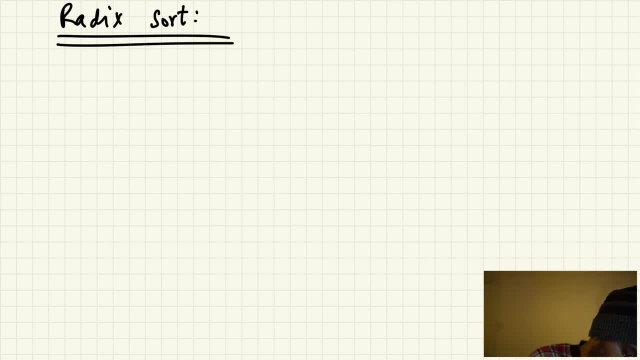 Let's say I'm given an array something like this: given 29,, 83,, 471,, 36,, 91 and 8. I want to sort this array. So what radix sort does is it's going to? we're going to use count. 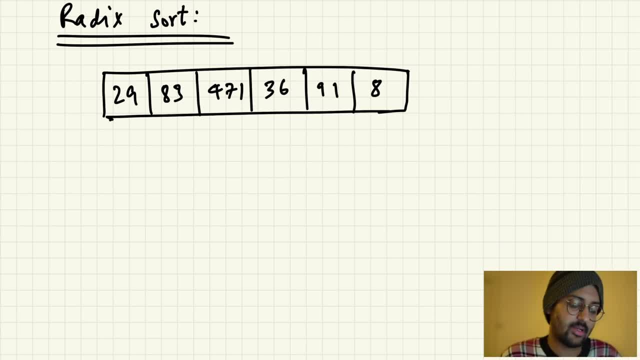 sort as well. But what radix sort does is? it's very simple. It divides the numbers into buckets and it sorts it according to those buckets, right based on every digit's value. So it's very simple. It's not confusing at all. This is one of the most easiest algorithms. Let me tell you what I mean. 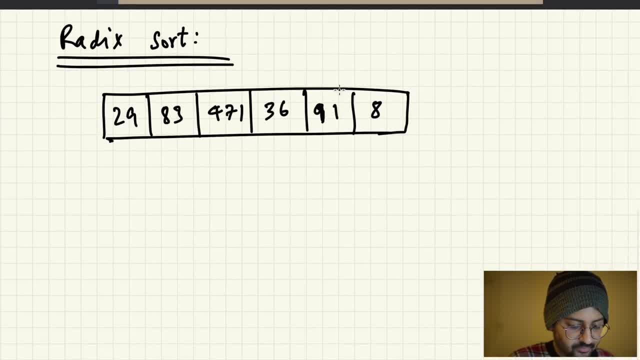 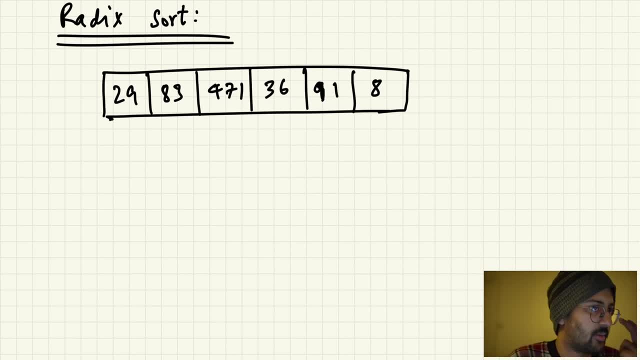 by buckets. So initially it's going to take the largest number, okay, the one with the most number of digits. So the first number has two digits. second number has two digits, eight and three. third number has three digits: 471 and then 221.. So largest number of digits in: 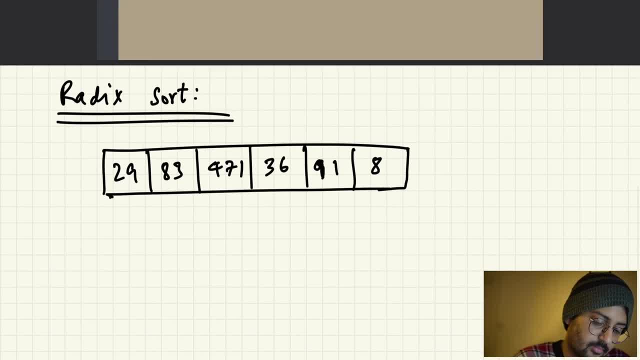 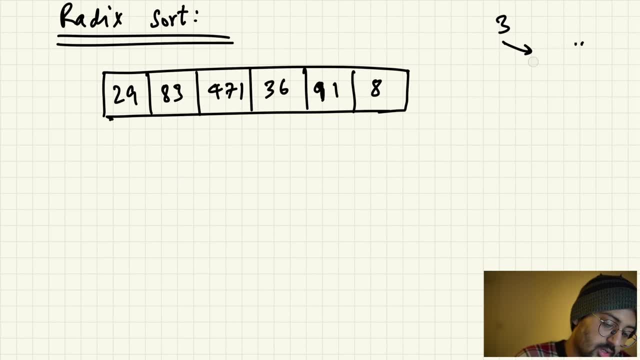 this array for any number is three. Hence I will run it three times. I will run, count, sort three times. For example, I can say largest digit is equal to three. run, count, sort three times. Okay, and it's going to run on the basis of the base values. So you know, in the childhood we have done base 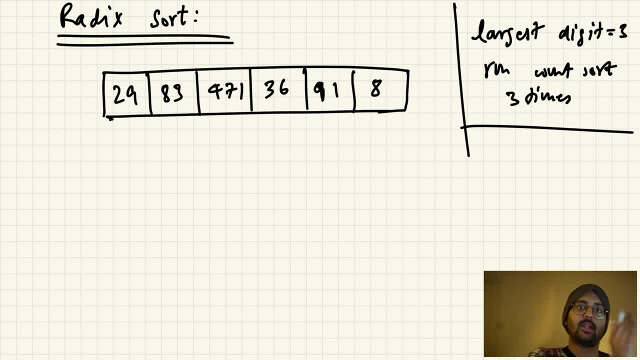 system: ones, tens, 100,000,, 10,000.. We are going to start from the least base and the least base and we'll work our way up, So from the zero, one, two, so ones place, tens, hundreds thousands, so on and so forth. So we will sort. 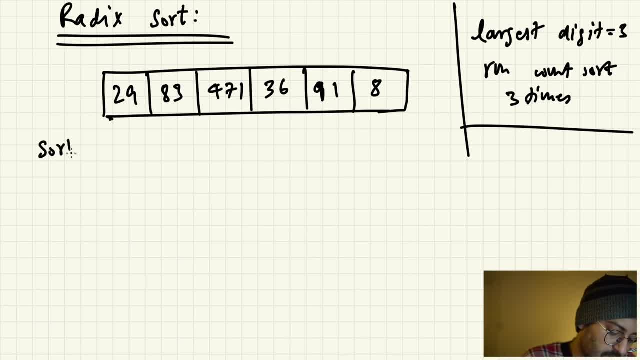 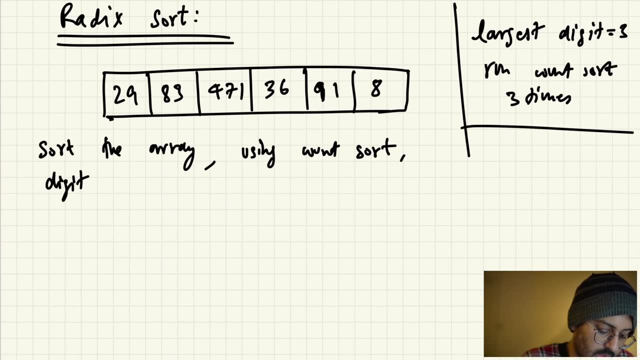 this array. Sort the array using count. sort digit by digit, starting from least. So least digit is what 0s 0th place. So I will sort it according to the 0th place, So 29,, 83,, 471,, 36,, 91, 8.. What is the least digit? This? 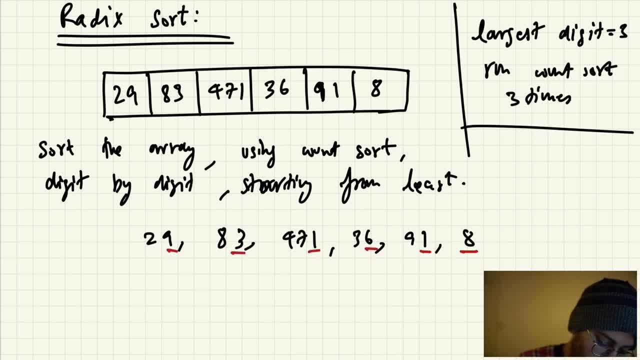 one, this one, All the 1s will be highlighted, the 1s place. Now I will sort it according to this. So if I sort it accordingly, first I will have, let's say, 471,, 91, and then. 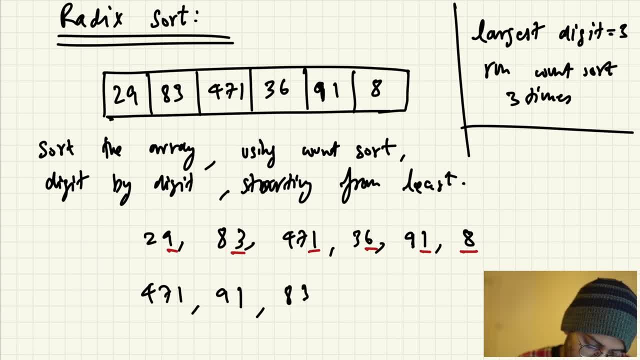 83,, 36,, 8, and 29.. You can see 1,, 1,, 3,, 6,, 7,, 8,, 9,, 10,, 11,, 12,, 13,, 14,, 15,, 16,, 17,, 18,. 19,, 20,, 21,, 21,, 22,, 23,, 24,, 25,, 26,, 27,, 28,, 29,, 30,, 31,, 32,, 33,, 34,, 35,, 36,, 37,, 38,, 39,. 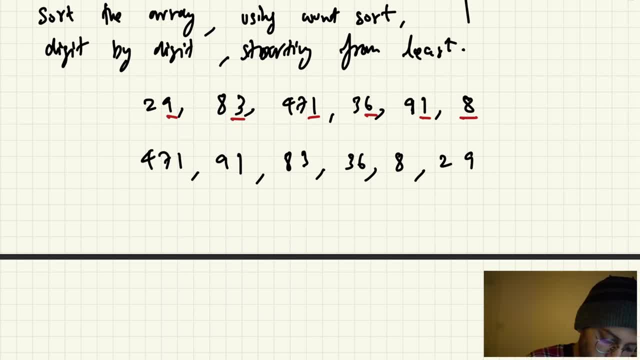 40. So 1, 1,, 3,, 6,, 8, 9.. Now what we're going to do is we're going to sort it again based on the next digits place. What comes after 1? 10th, 10th digit place, So 10th. 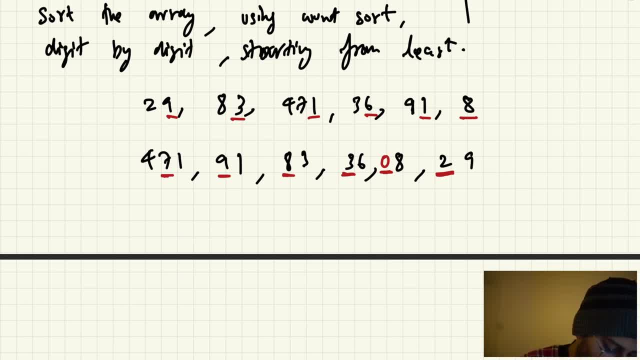 digit place. here is 2.. Here is 0.. Here is 3,, 8,, 9, and 7.. Now sort it. So there you: 0, 8, 8 will be coming first, then I will have 29, then I will have 36, then I will. 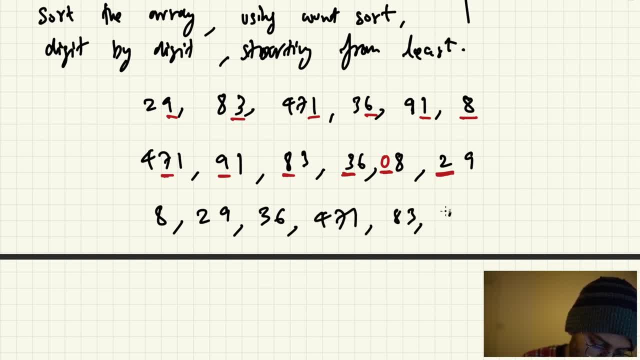 have 471, then 83 and then 91. now I will sort accordingly. so this you can see how I'm doing every since at every loop I am sorting the array based on the single digit. it means that these red red things will be from 0 to 9, only red digits only. 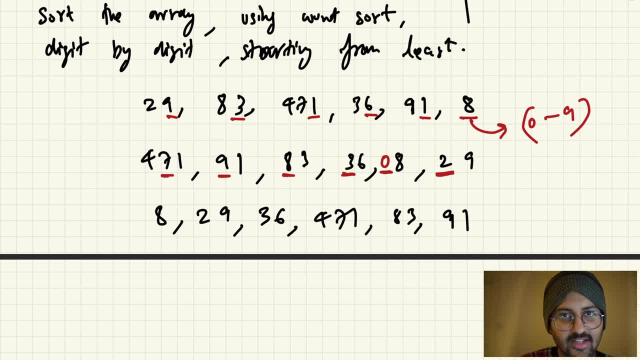 one digit right we are solving right. and how many one digit numbers are there in the world? 10, 0 to 9, so we can use count sort at every level and this is going to run how many times number of times we have the largest digits. obviously makes 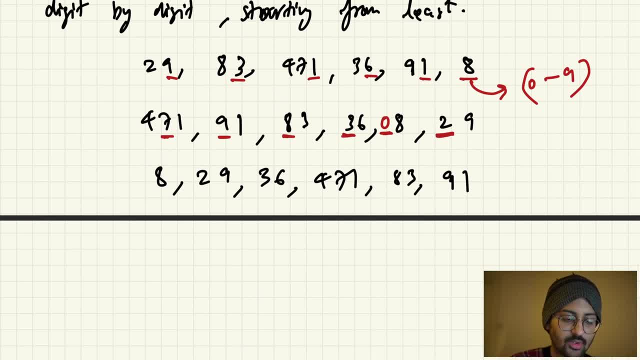 sense you can't run it four times because there is no fourth place, no thousands place. now it will be like: okay, now at the third next turn, index: 0 0, 4, 0, 0, 0. so it will become. it will become 8, 29, 36, 83, 91, 471. 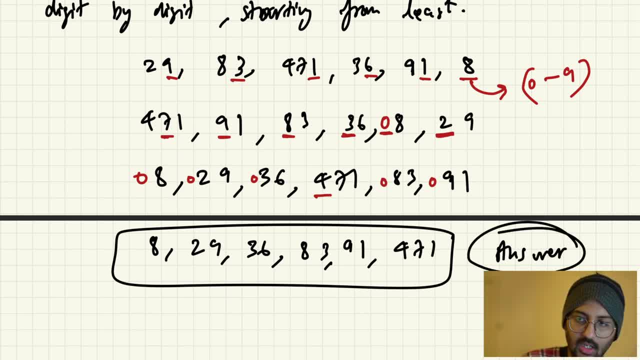 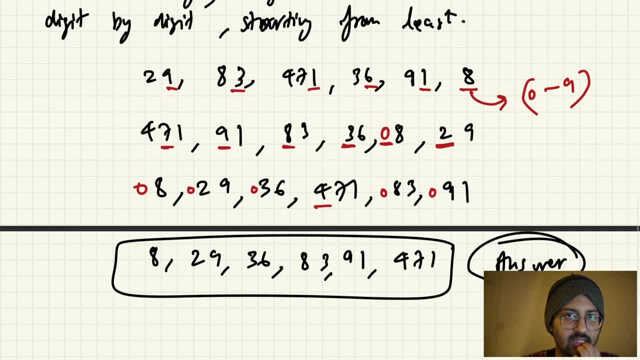 this is my answer. array sorted answer. array sorted, simple. so calculate the number, largest number of digits, run, count, sort that many times. that's it. and every time you run, count, sort, run it for the index starting from the left hand side. so 0th index. so 0, 0th place, like ones place. 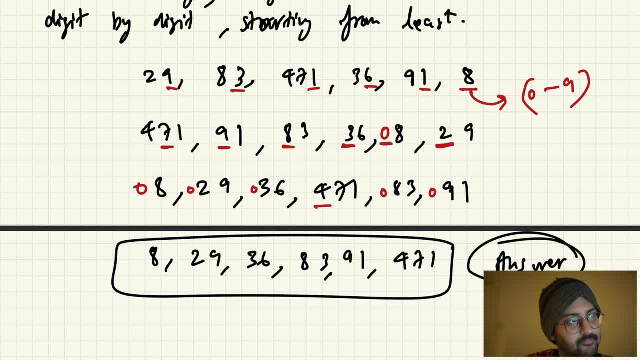 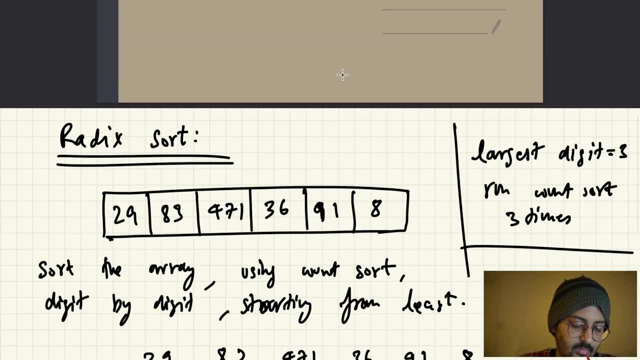 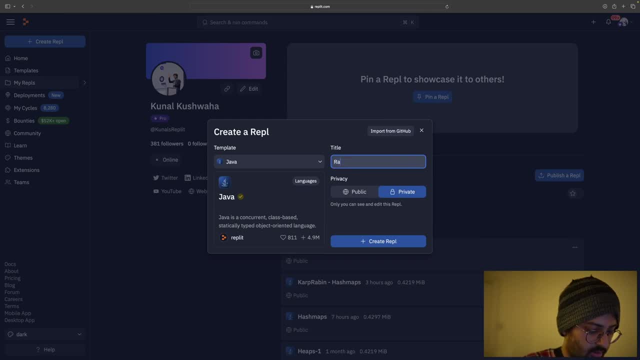 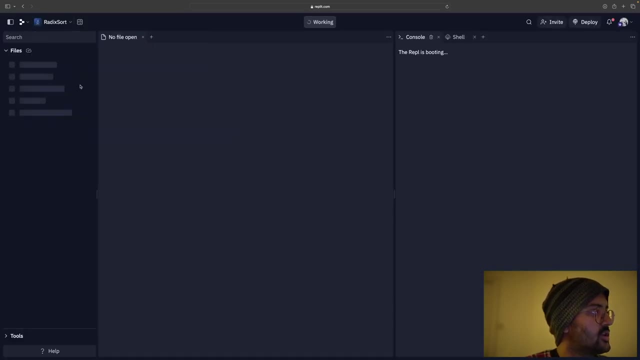 tens place, hundreds plates, thousands place. that's it, okay. I'll talk to about the time, complexity and the advantages and stuff later on. but let's code it and it's pretty simple, okay, so the link can be found in the description below. I will call it radix sort. I'll make it public so you can check it out and what. 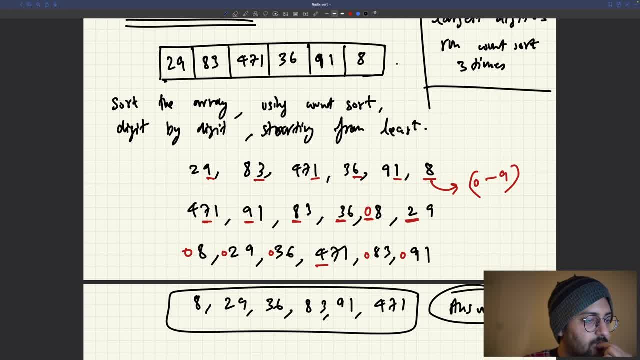 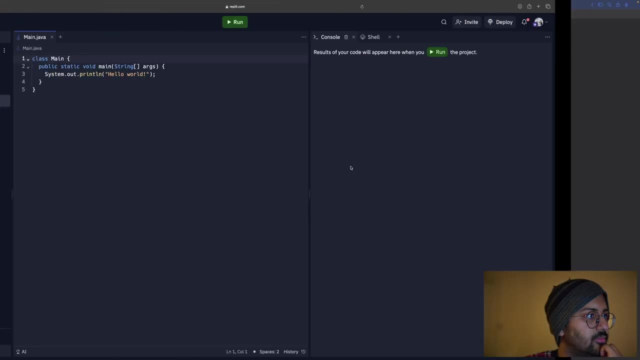 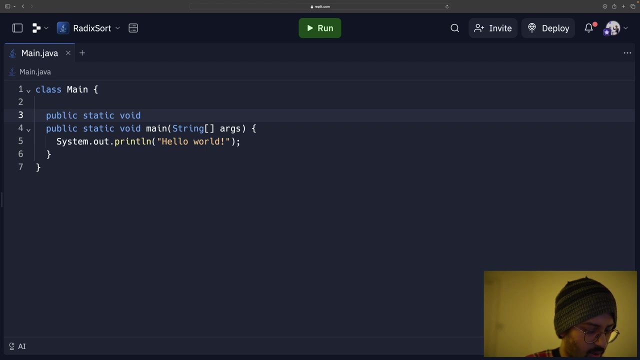 are we going to do? how are we going to do this? first I'm going to calculate the maximum number of digits, right, and then I'm going to check that count sort for every digits place, right. and that's what we're going to do. so I'm going to say: public static void radix sort. 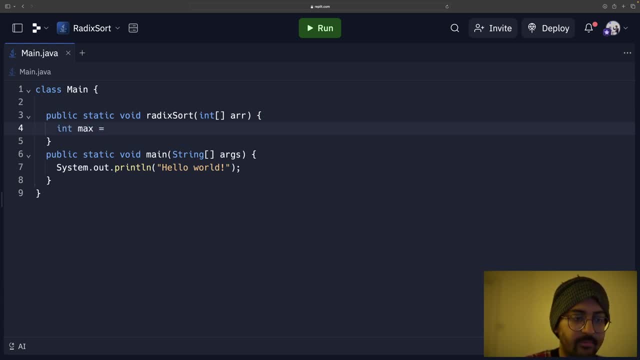 int array. I want to get the maximum number first to do the number of digits. that's what the number of digits will be. maximum number, so maximum number. I can get arrays dot stream. you can also do a simple linear search. if you want max dot, get as int. 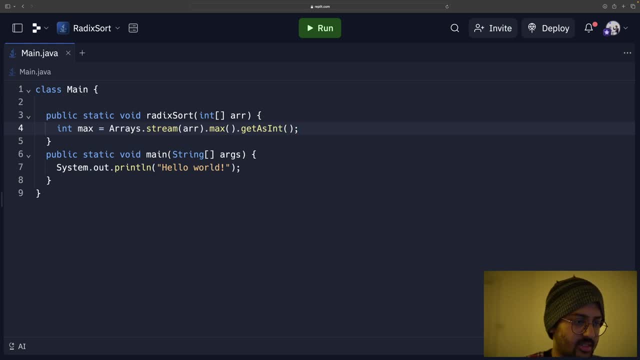 okay, and I've shown you the formula to calculate the number of digits previously as well, so nothing to worry about it. now I'm going to say: do count, sort for every digit place, starting from once, once, then tens, then hundred, then thousand and ten thousand, so exp. 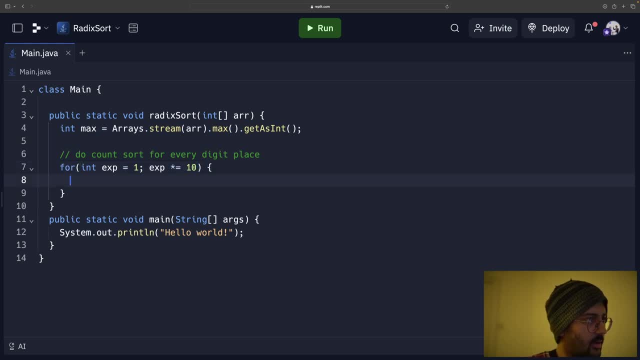 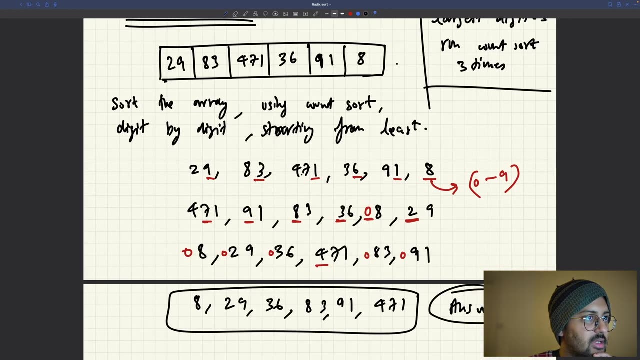 multiplied by 10 at every step. but what is the condition? how? how long will it go? let's say we have 471, so that is the largest number: 471, experience exp. my exponent will be 1, then my exponent will be 10, then my exponent will be 100, then I don't want it to be thousand, so this: 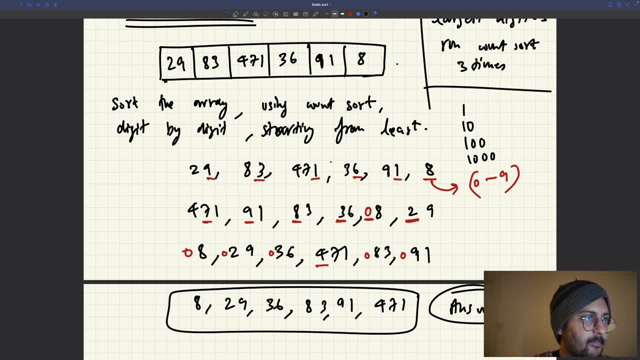 exponent. so my number modulo exponent should be positive or greater than 0. see, because if I am at 1, I know that 1 modulo like the number modulo 1, which is 471. so if I am at 1, I know that 1 modulo like the number modulo 1, which is 471. 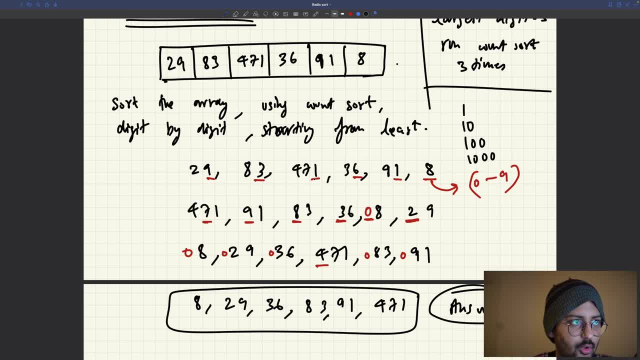 so if I am at 1, I know that 1 modulo 1, which is 471 remainder 1, like divided by like 471 remainder 1 like divided by like 471 remainder 1, like divided by like modulo 1, not not remainder, divide 471. 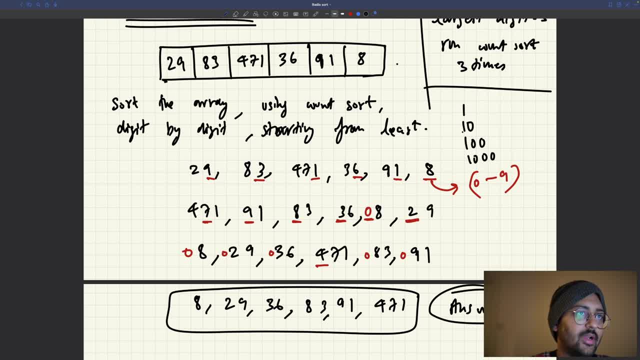 modulo 1, not not remainder divide. 471 modulo 1, not not remainder divide. 471 divided by 1 is 471, so I think this will: divided by 1 is 471. so I think this will, divided by 1 is 471. so I think this will work. then I will go with tens place does. 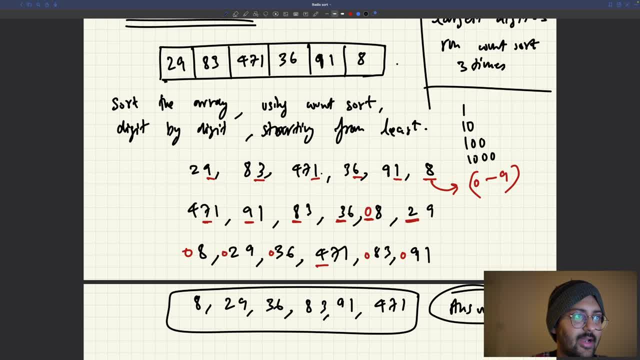 work, then I will go with tens place. does work, then I will go with tens place. does it have a tens place? yes, it does because it have a tens place. yes, it does because it have a tens place. yes, it does because 471 divided by 10 is giving me a. 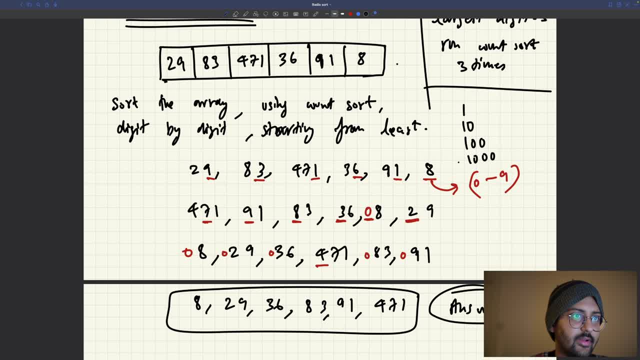 471 divided by 10 is giving me a. 471 divided by 10 is giving me a positive number. right 47, then it will be positive number. right 47, then it will be positive number. right 47, then it will be 100. because for like I can say: 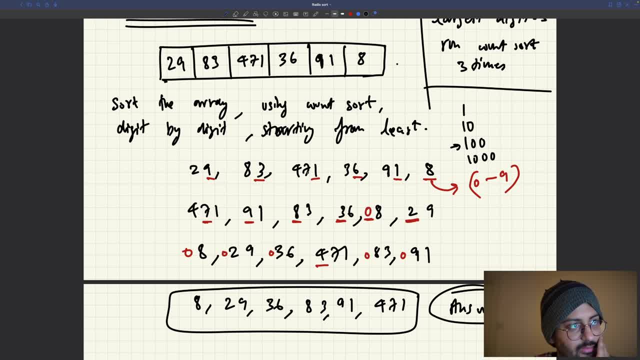 I can say that 471 divided by 100 is. I can say that 471 divided by 100 is. I can say that 471 divided by 100 is. giving me a positive number, say a 471. giving me a positive number, say a 471. 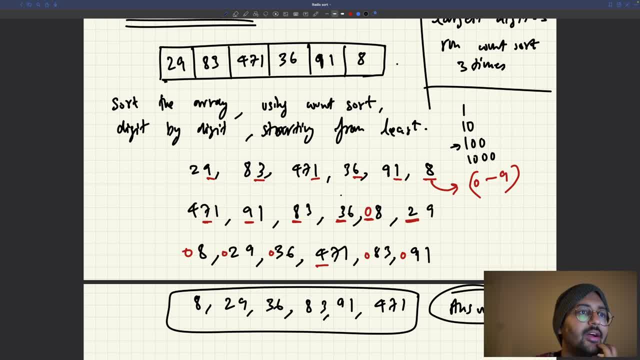 giving me a positive number, say a 471 divided by 1, 471 divided by 10, 471 divided by 1, 471 divided by 10, 471 divided by 1, 471 divided by 10, 471 divided by 100, and then 471 divided by: 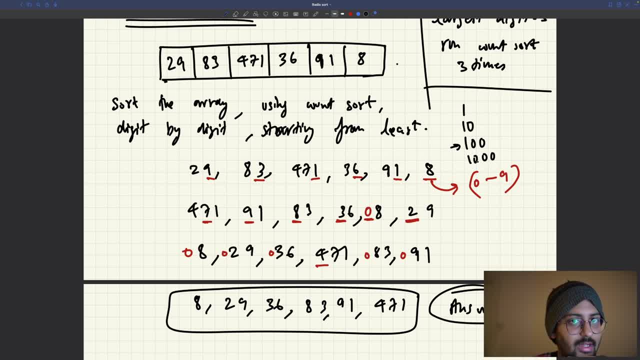 divided by 100 and then 471 divided by. divided by 100 and then 471 divided by 1000. it's giving me not equal 1000. it's giving me not equal 1000. it's giving me not equal, not greater than 0. so I cannot take. 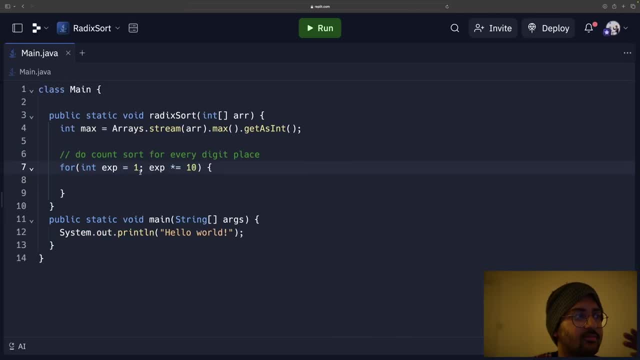 not greater than 0, so I cannot take. not greater than 0, so I cannot take thousand. or you can also just run it thousand, or you can also just run it thousand, or you can also just run it. number of times the you know the number. number of times the you know the number. 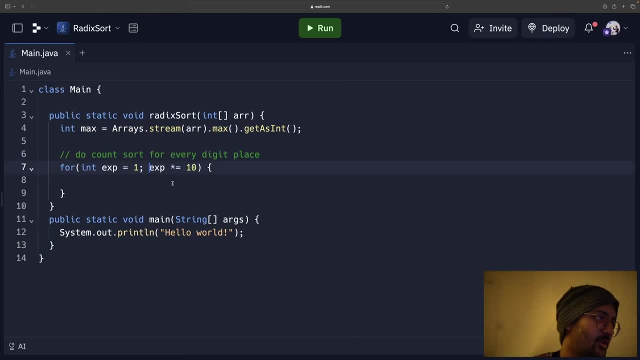 number of times the you know the number of digits are. using the log, you can find of digits are using the log, you can find of digits are using the log, you can find digits log 10 something log base 2, or digits log 10 something log base 2 or. 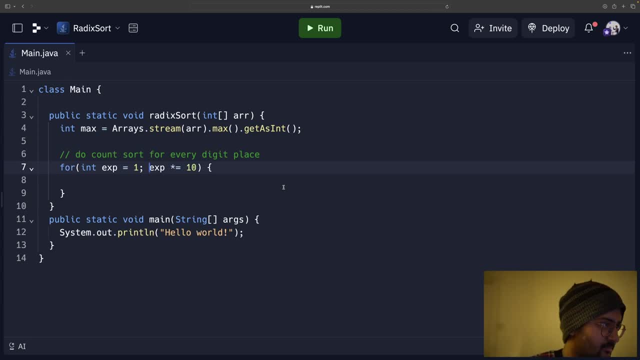 digits, log 10 something, log base 2 or something. I've covered it in the math for something. I've covered it in the math for something. I've covered it in the math for CS classes. but anyway, I'll do nice one, CS classes, but anyway, I'll do nice one. 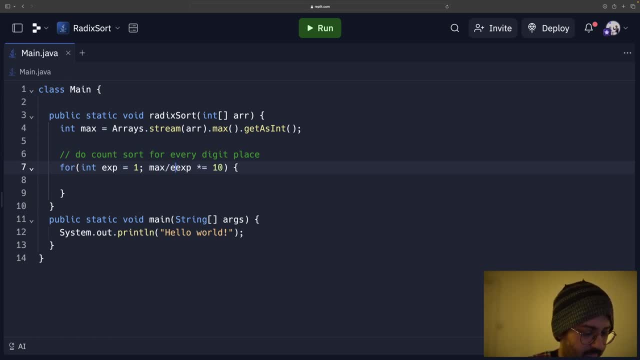 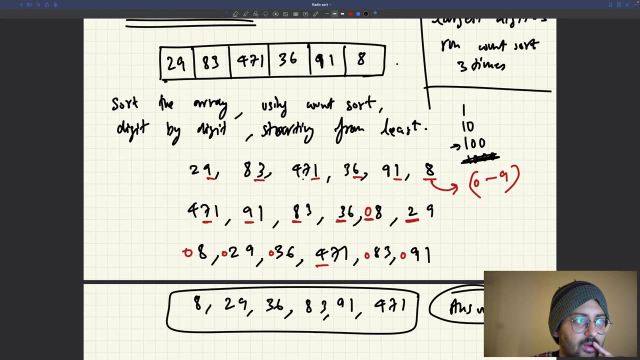 CS classes. but anyway, I'll do nice one. nice way: max divided by exponent. nice way. max divided by exponent. nice way: max divided by exponent should be greater than 0, so this will run. should be greater than 0, so this will run. should be greater than 0, so this will run three times for any number with three. 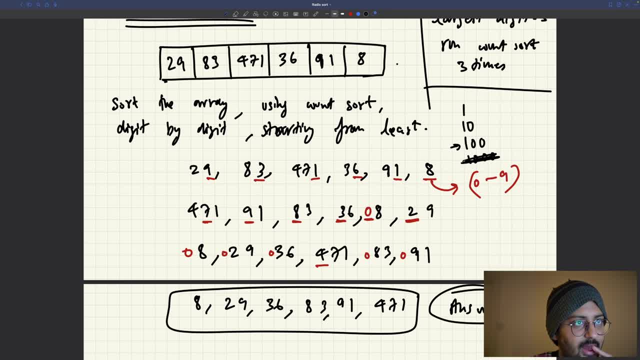 three times for any number with three. three times for any number with three digits. okay when it reaches the fourth digits. okay when it reaches the fourth digits. okay when it reaches the fourth time. it will be like okay thousand if time. it will be like okay thousand if. 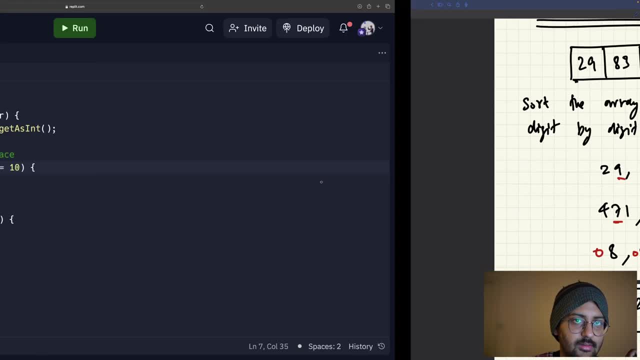 time it will be like: okay, thousand, if you number, divide this number by you number, divide this number by you number, divide this number by thousand. I'm getting you know it's thousand. I'm getting you know it's thousand. I'm getting you know it's getting zero and stuff. I want it to be. 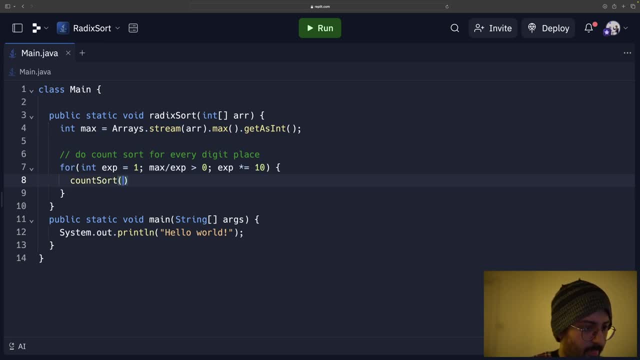 getting zero and stuff I want it to be getting zero and stuff I want it to be greater than zero. do count, sort count greater than zero. do count sort greater than zero. do count, sort count. sort of this area for this exponent: okay. sort of this area for this exponent: okay. 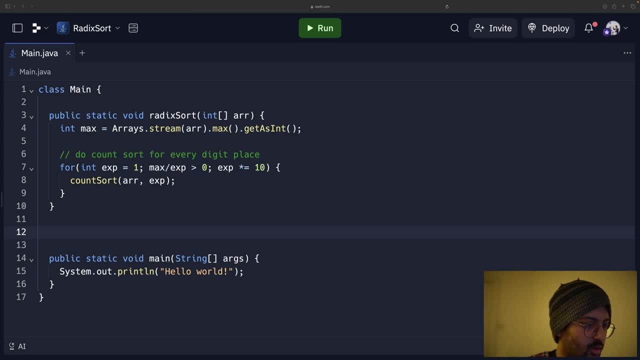 sort of this area for this exponent. okay, let's do count sort so for count sort. let's do count sort so for count sort. let's do count sort so for count sort. it's going to be very simple, I'm going. it's going to be very simple, I'm going. 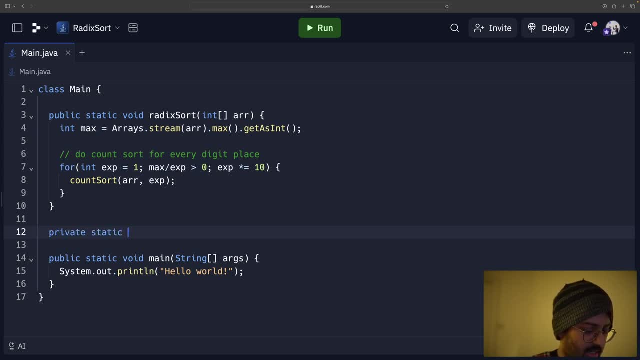 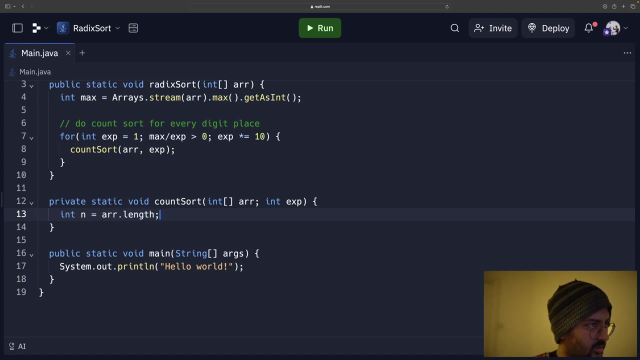 it's going to be very simple. I'm going to say private static void count. sort. to say private static void count. sort to say private static void count sort. int array. int array. int array. my exponent just gonna make some. my exponent just gonna make some. my exponent just gonna make some variables. array dot length. 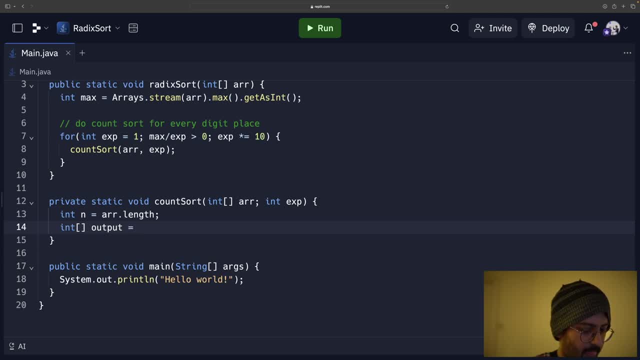 variables array dot length. variables array dot length. I'll have my output array- new int n and I'll have my output array- new int n and I'll have my output array- new int n and my count array, which is going to be my count array, which is going to be. 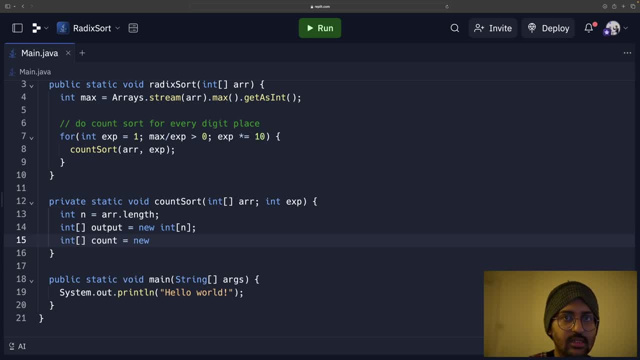 my count array which is going to be equal to of what size size? 10 because 0 equal to of what size size 10 because 0. equal to of what size size 10 because 0 to 9 10 numbers. okay, you can initialize. 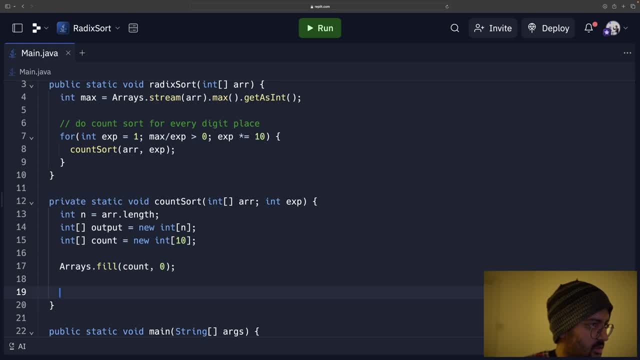 to 9- 10 numbers. okay, you can initialize to 9- 10 numbers. okay, you can initialize it all with 0, but I think by default is it all with 0. but I think by default is it all with 0, but I think by default is already 0. so it's fine, and now I'm. 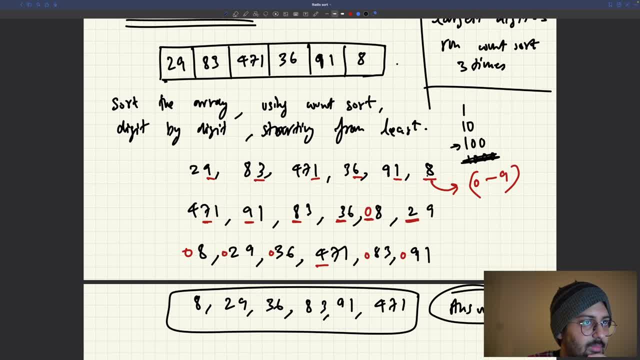 already 0, so it's fine. and now I'm already 0, so it's fine. and now I'm gonna do for. let's say, if I am at exponent gonna do for. let's say, if I am at exponent gonna do for. let's say, if I am at exponent 1. so I need to make a frequency. 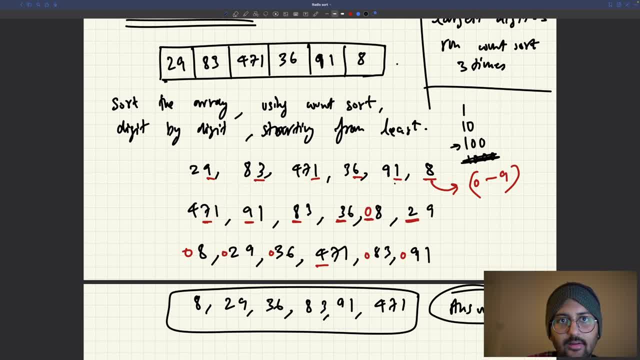 1. so I need to make a frequency 1. so I need to make a frequency array of all the numbers at index, like the bit array of all the numbers at index, like the bit array of all the numbers at index, like the bit place of 1. so 1 stands 100, so how? 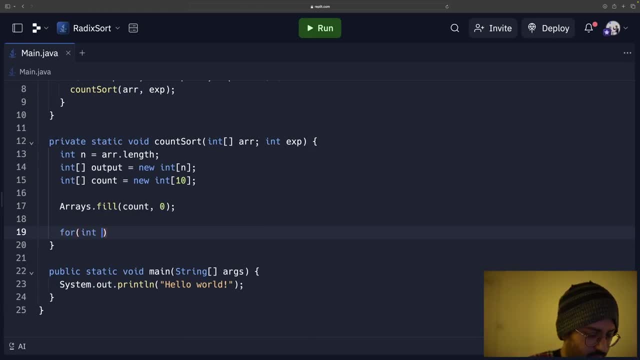 place of 1, so 1 stands 100. so how? place of 1, so 1 stands 100. so how can I do that? I know I will do. I is equal to. can I do that? I know I will do. I is equal to. can I do that? I know I will do. I is equal to 0, I is less than n, so I will. 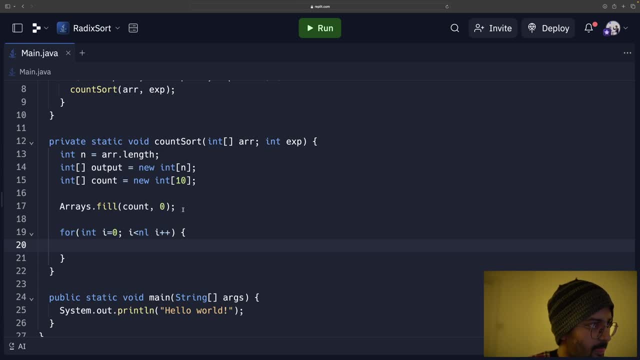 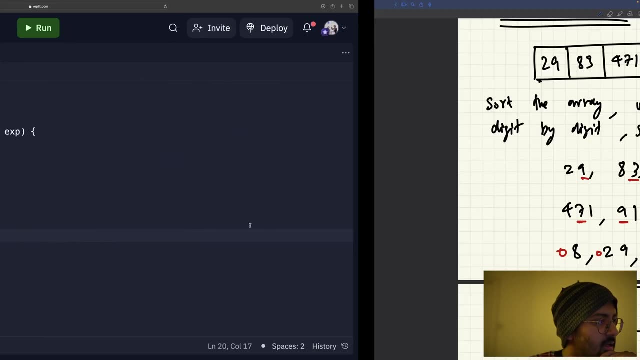 0 I is less than n, so I will 0- I is less than n, so I will traverse through all the elements and I traverse through all the elements, and I traverse through all the elements and I plus plus. I want to make the count array. okay, I want to do count of something plus plus. now, what would that? something? 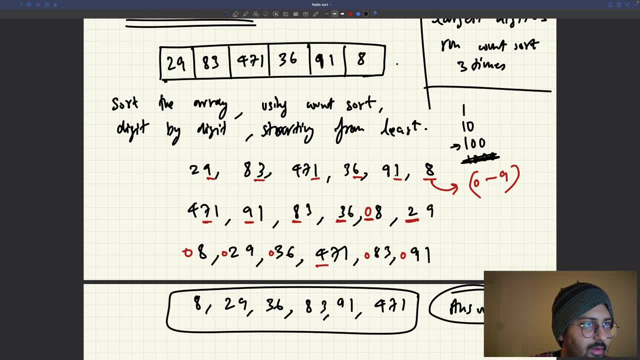 okay, I want to do count of something plus plus. now, what would that something be? how do I get 8, 1, 6? it will be: whatever element I am at here I need to get. so if I'm at, let's say this. second one I want to get to exponent here is 10. 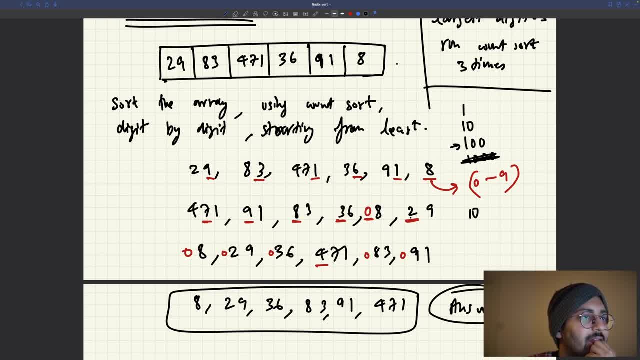 I want to get to exponent. here is 10. how do I get to? I can say 20. how do I get to? I can say 20. how do I get to? I can say 20. 9 divided by remove all the elements on. 9 divided by remove all the elements on. 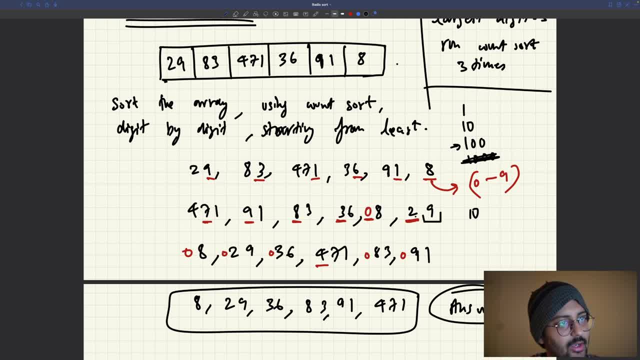 9 divided by: remove all the elements on the right-hand side so that I can do why the right-hand side, so that I can do why the right-hand side, so that I can do why 29 divided by 10, so 29 divided by 10 will. 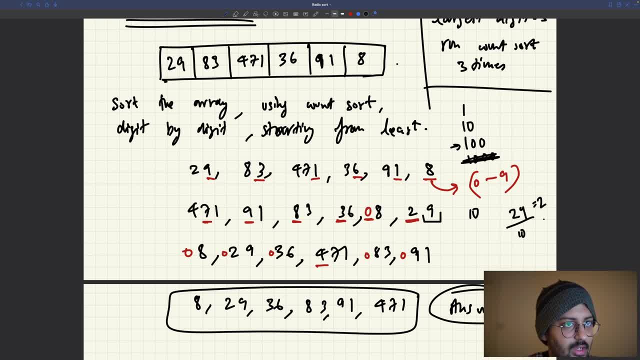 29 divided by 10, so 29 divided by 10 will 29 divided by 10, so 29 divided by 10 will give me 2 and then just take the give me 2 and then just take the give me 2 and then just take the remainder, whatever the last element is. 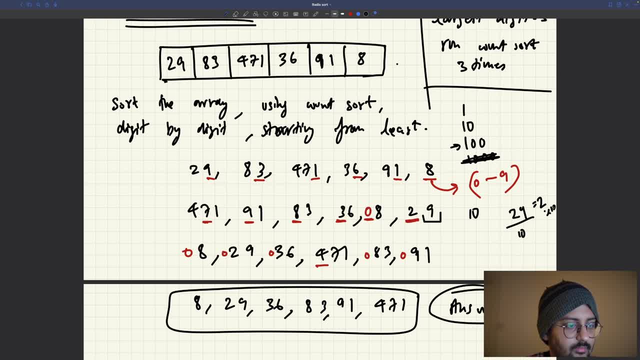 remainder. whatever the last element is remainder. whatever the last element is, that can be modulo 10, that can be modulo 10. that can be modulo 10. okay easy, I hope you are able to. okay easy, I hope you are able to. okay easy. I hope you are able to understand. let me show you. so let's say: 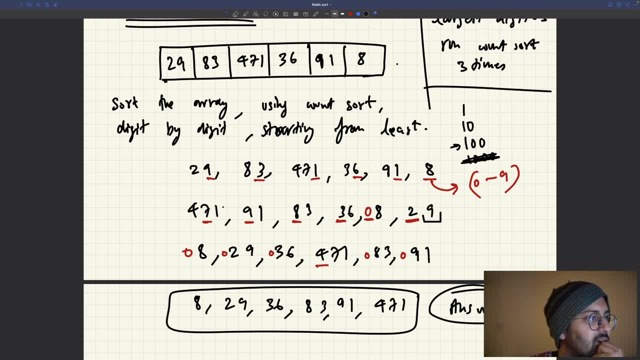 understand. let me show you. so let's say: there is a number, let's say 471 and I. there is a number, let's say 471 and I. there is a number, let's say 471, and I want to get 7 at exponent number 10. I'm. 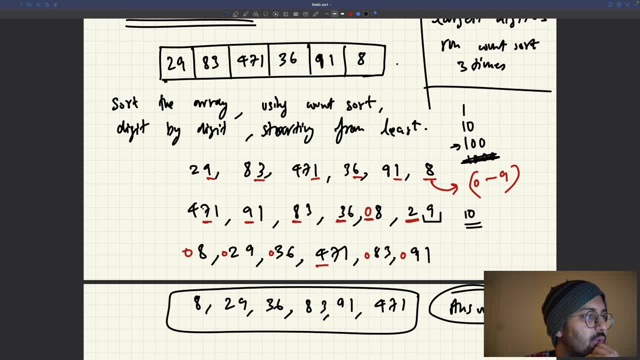 want to get 7 at exponent number 10. I'm want to get 7 at exponent number 10. I'm doing the loop for exponent number 10, so doing the loop for exponent number 10, so doing the loop for exponent number 10. so how would I get 7? remove all the ones on. 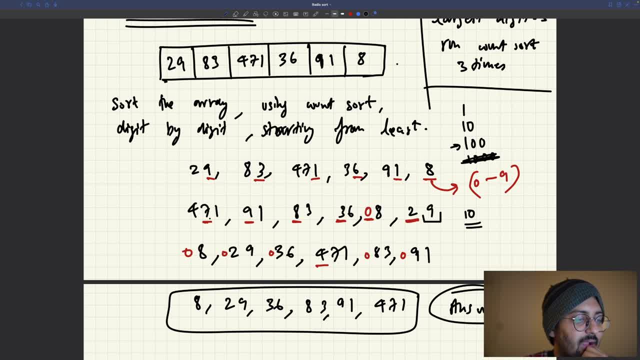 how would I get 7? remove all the ones on. how would I get 7? remove all the ones on the right-hand side. so divided by 10, the right-hand side, so divided by 10, the right-hand side. so divided by 10 means divided by exponent. it will give me. 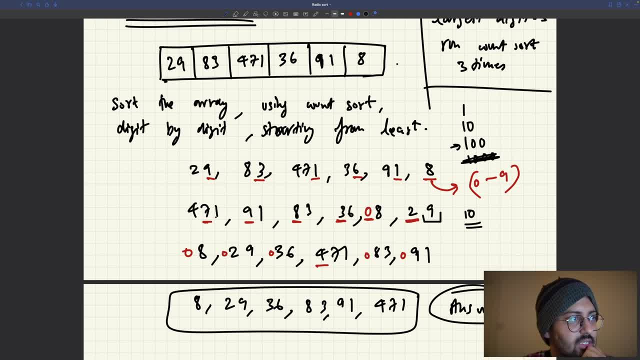 means divided by exponent. it will give me means divided by exponent. it will give me 47, and then the last digit, 47 modulo 10, 47, and then the last digit, 47 modulo 10, 47, and then the last digit, 47 modulo 10, will give me 7. similarly, 91 divided by 10. 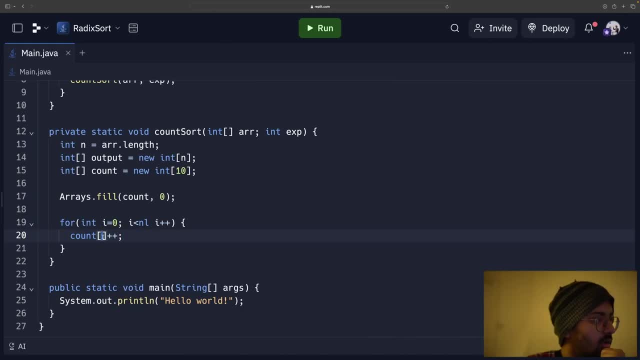 will give me 7, similarly 91, divided by 10. will give me 7, similarly 91, divided by 10: 9, last digit 9. so I will say array of I 9, last digit: 9. so I will say array of I, 9, last digit: 9. so I will say array of I divide by exponent, and then take the. 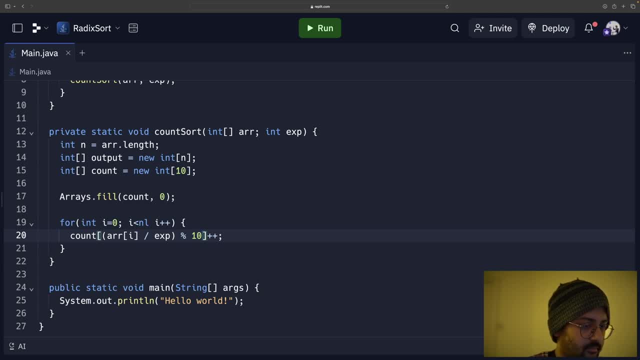 divide by exponent and then take the divide by exponent and then take the model over 10. okay, sounds good. okay now. model over 10. okay, sounds good. okay now, model over 10. okay, sounds good, okay now. one thing is that some of these arrays. one thing is that some of these arrays. 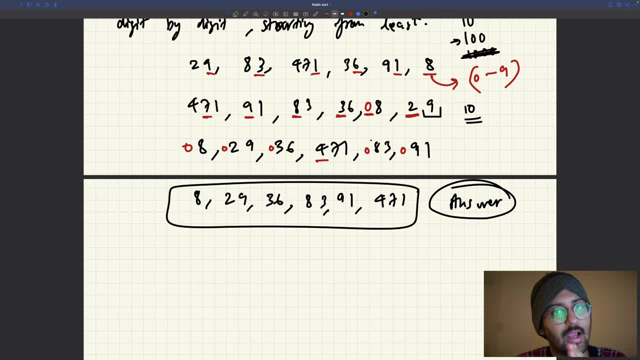 one thing is that some of these arrays now we'll have in the count array, from now we'll have in the count array. from now we'll have in the count array from 0 to 9 it will have some elements as 0: 0 to 9. it will have some elements as 0. 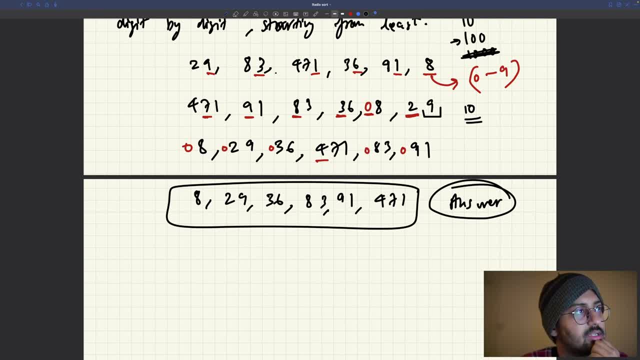 0 to 9. it will have some elements as 0. the question is: since I'm working with, the question is: since I'm working with, the question is: since I'm working with single digit numbers, how do I get the single digit numbers? how do I get the? 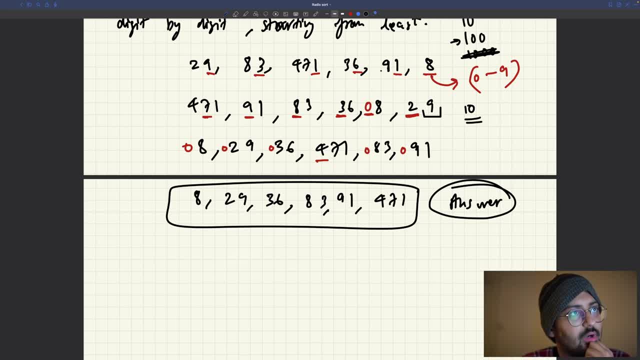 single digit numbers. how do I get the original numbers? because in reality I'm original numbers, because in reality I'm original numbers, because in reality I'm sorting the original numbers right. so sorting the original numbers right, so sorting the original numbers right. so what I'm going to do is I'm just gonna 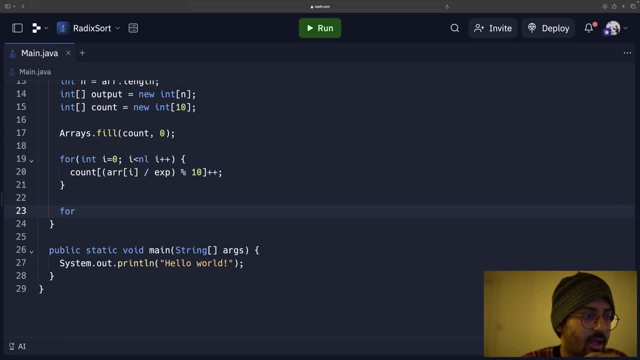 what I'm going to do is I'm just gonna. what I'm going to do is I'm just gonna build, like change the every element of build. like change the every element of build. like change the every element of count of I, so that count of I also. 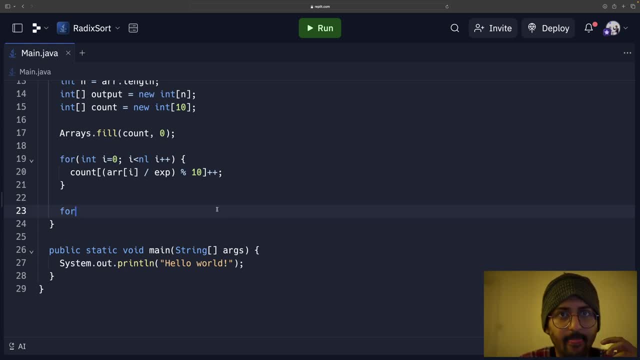 count of I, so that count of I also count of I so that count of I also contains the actual position of the. contains the actual position of the. contains the actual position of the digit in the in the output array that digit in the in the output array that. 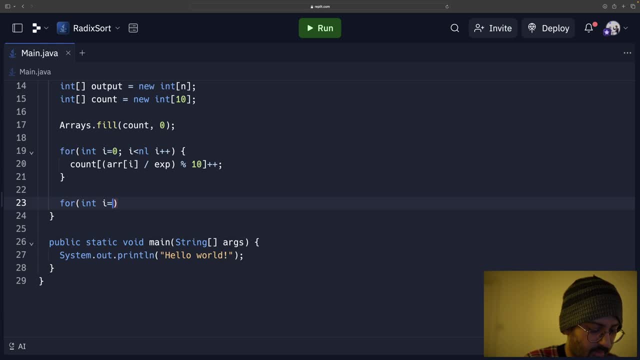 digit in the, in the output array, that we'll create. let me show you, I'll just, we'll create. let me show you, I'll just, we'll create. let me show you, I'll just, I'll just do one thing, so in I is equal. I'll just do one thing, so in I is equal. 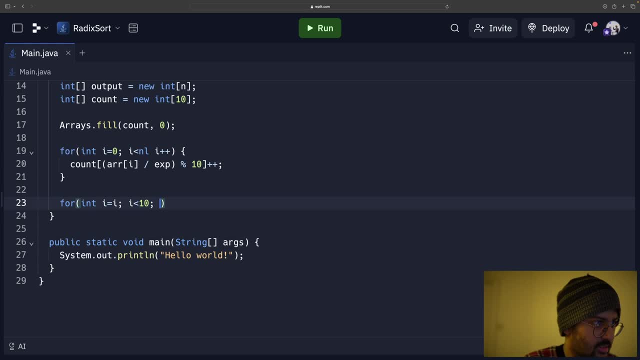 I'll just do one thing. so in: I is equal to 1. I is less than our 10 research the to 1. I is less than our 10 research the to 1. I is less than our 10 research the till till 9. I will go and I will say: 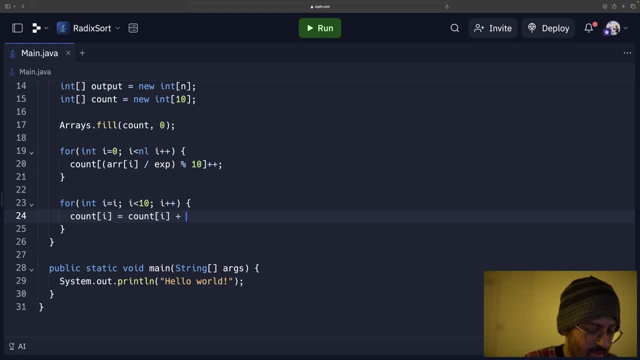 till till 9, I will go, and I will say till till 9, I will go, and I will say: count of I is equal to count of I, plus count of I is equal to count of I, plus count of I is equal to count of I plus the previous one, count of I minus 1 I. 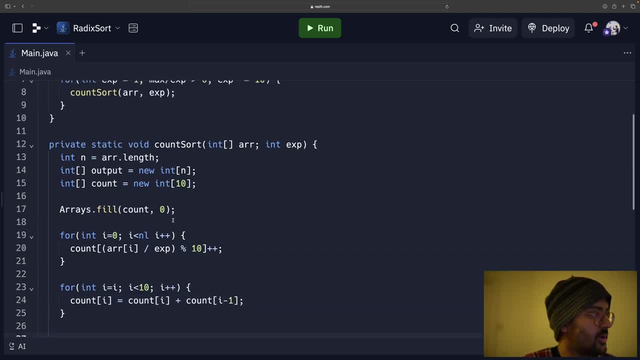 the previous one count of I minus 1. I the previous one count of I minus 1. I will show you what I did, so what I'm will show you what I did, so what I'm will show you what I did. so what I'm going to do is I'm going to actually 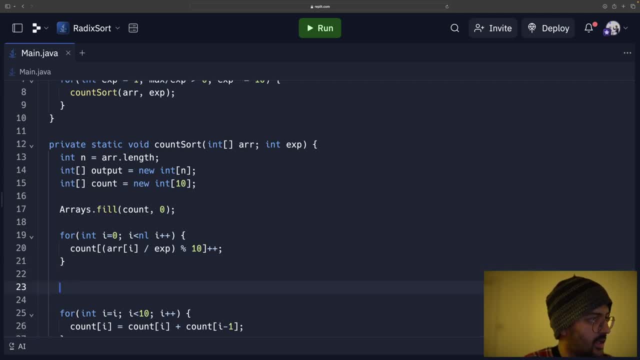 going to do? is I'm going to actually going to do? is I'm going to actually print at every step? okay, so at here, I print at every step. okay, so at here, I print at every step. okay, so at here I will print. system dot out, dot print Ellen. 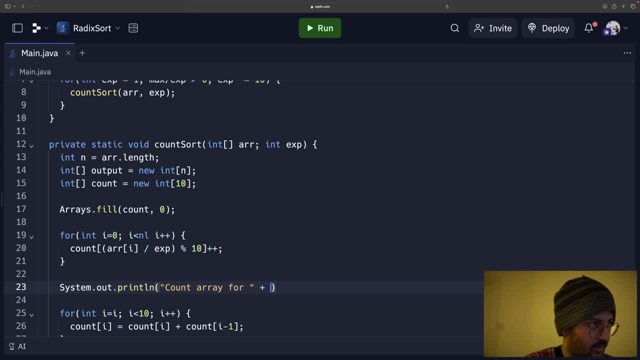 count array, for I'm just printing it so you can see at. I'm just printing it, so you can see at. I'm just printing it, so you can see at every level what is happening, and then every level what is happening, and then every level what is happening, and then I'll be able to show you why I'm doing. 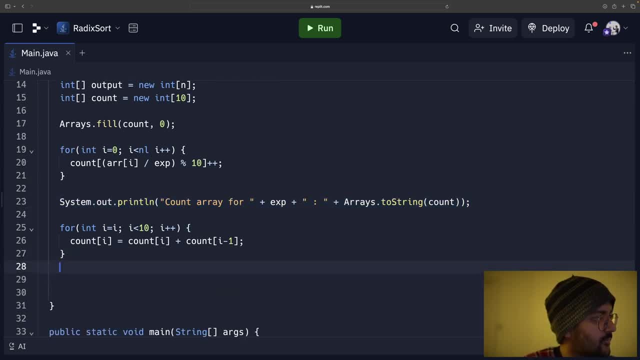 I'll be able to show you why I'm doing. I'll be able to show you why I'm doing what I'm doing. okay, so this is the count what I'm doing. okay, so this is the count what I'm doing. okay, so this is the count array. 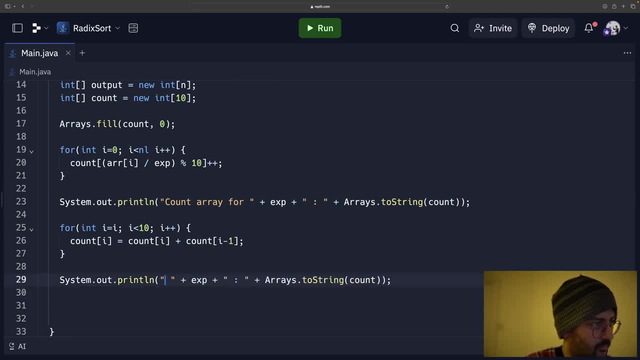 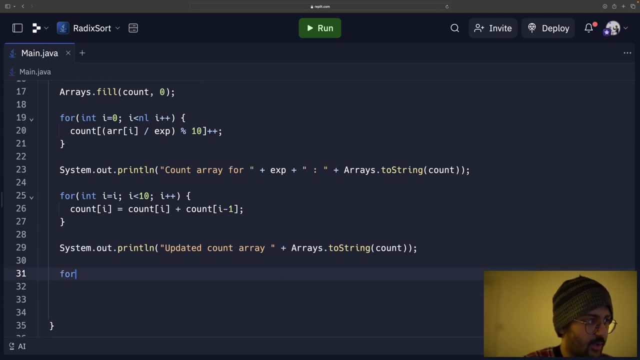 array array. updated count array. updated count array. now I will build the output array. okay, now I will build the output array. okay, now I will build the output array. okay, so I will say for if I'm saying the. so I will say for if I'm saying the. 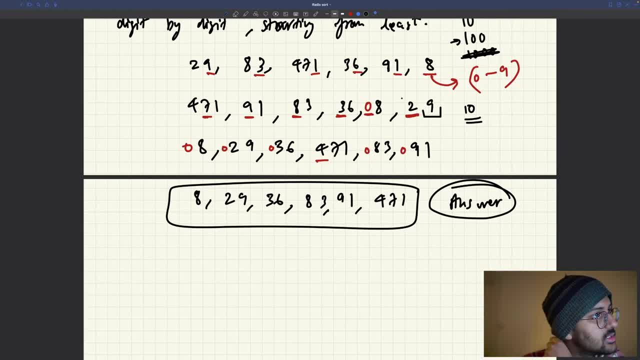 so I will say: for if I'm saying the output array means I have to have the output array means I have to have the output array means I have to have the original item. let's say if this is index, original item. let's say if this is index. 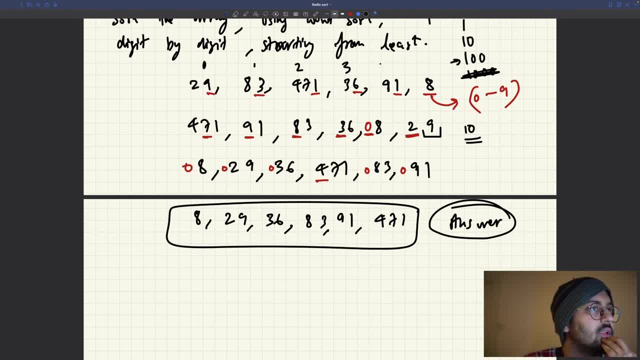 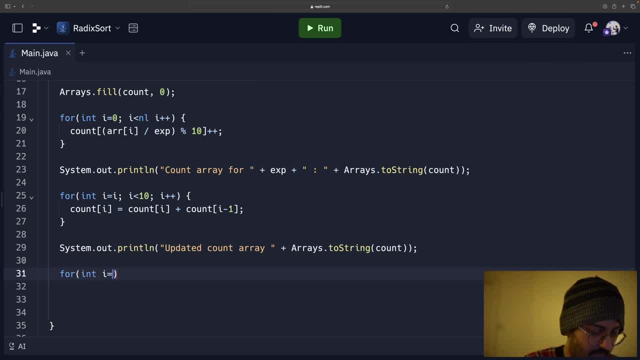 original item. let's say, if this is index, number zero one, two, three, four, five and number zero one, two, three, four five and number zero one, two, three, four, five. and I made it account so I can say for in tie. I made it account so I can say for in tie. 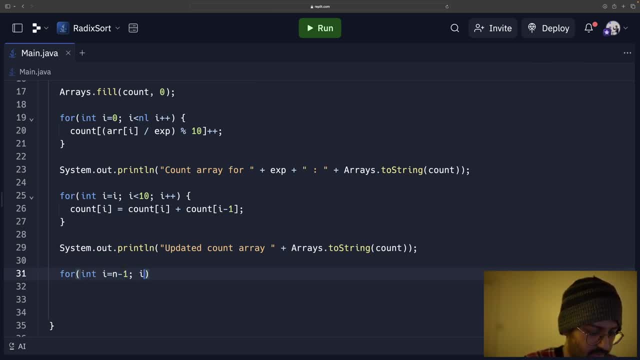 I made it account so I can say for in tie. just bear with me, for a second in tie is just bear with me. for a second in tie is just bear with me, for a second in tie is equal to n minus 1. I is greater than. 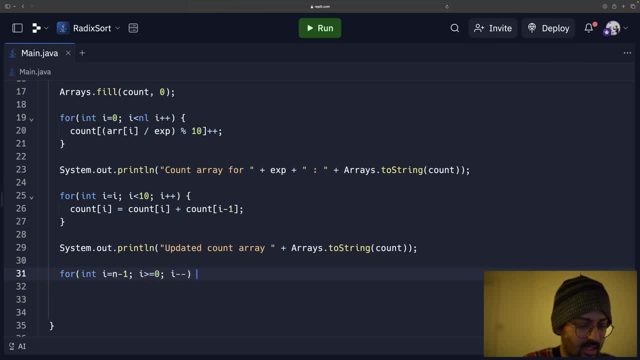 equal to n minus 1. I is greater than equal to n minus 1. I is greater than equal to 0 and I minus minus, I will start equal to 0 and I minus minus, I will start equal to 0 and I minus minus, I will start from the very end and I will say that. 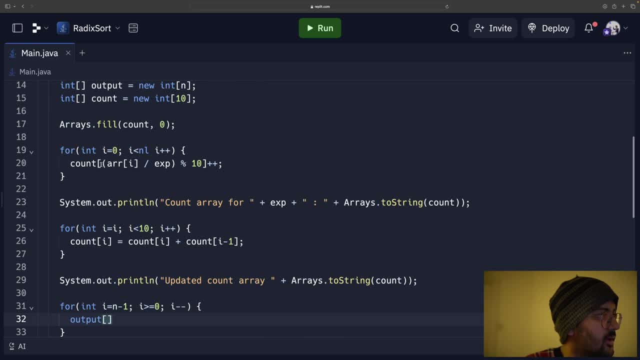 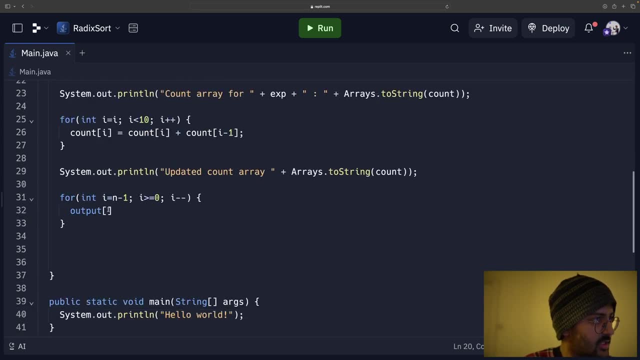 from the very end, and I will say that from the very end, and I will say that the output of the same, the output of the same, the output of the same. count of air RFI exponent percentage: 10. so count of air RFI exponent percentage: 10. so 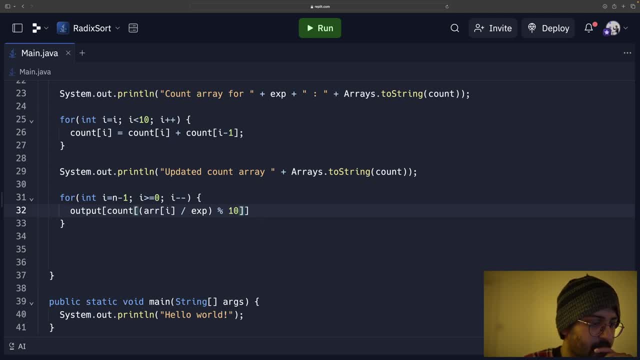 count of air RFI exponent percentage: 10. so the output of this, the output of this, the output of this, okay at this index is going to be equal. okay at this index is going to be equal. okay at this index is going to be equal to what? not a RR of I minus 1, because 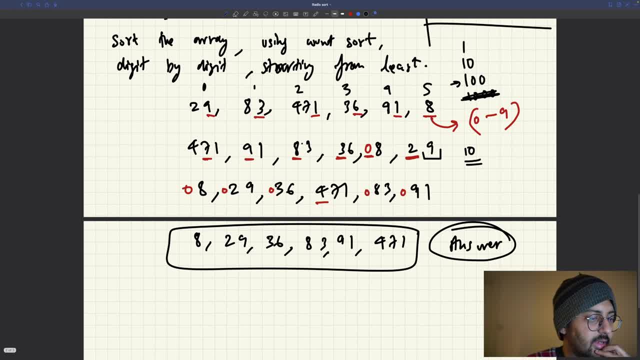 to what not a RR of I minus 1? because to what not a RR of I minus 1? because let me show you if I, if I just build it, let me show you. if I, if I just build it, let me show you. if I, if I just build it, let me show you, let me just write it. 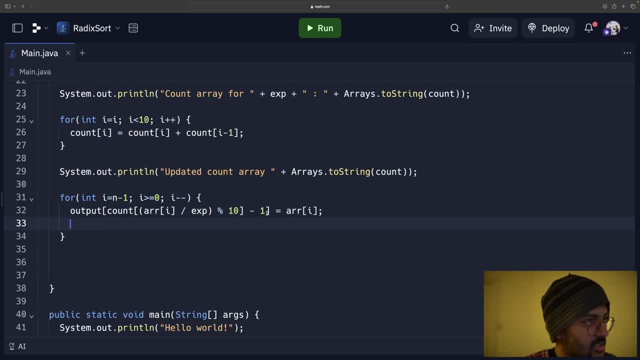 let me show you, let me just write it, let me show you, let me just write it down, and then I will show you and once down, and then I will show you, and once down, and then I will show you, and once this is taken, like one element is taken, 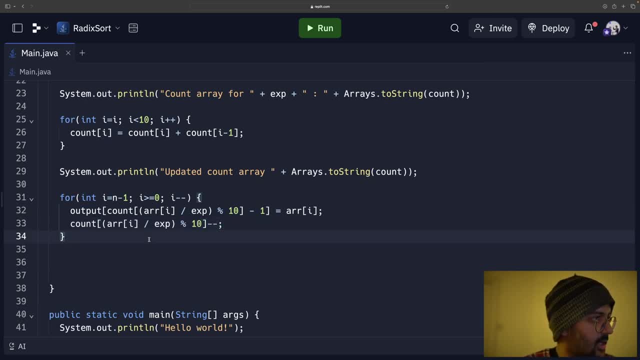 this is taken like one element is taken. this is taken like one element is taken: it will be minus, minus, and then in the, it will be minus, minus, and then in the, it will be minus, minus, and then in the end, or after every single step, the array. 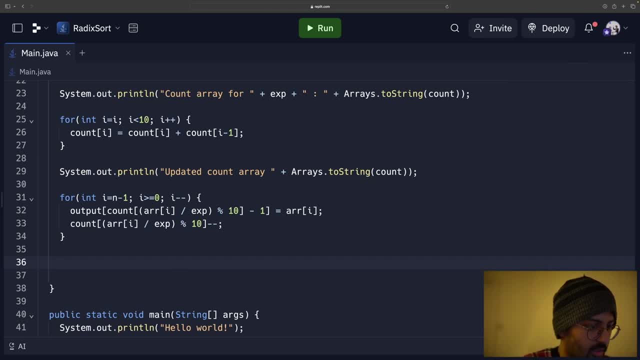 end or after every single step. the array end or after every single step. the array is being sorted, so just replace the is being sorted, so just replace the is being sorted, so just replace the output with the main one. okay, and I will output with the main one. okay, and I will. 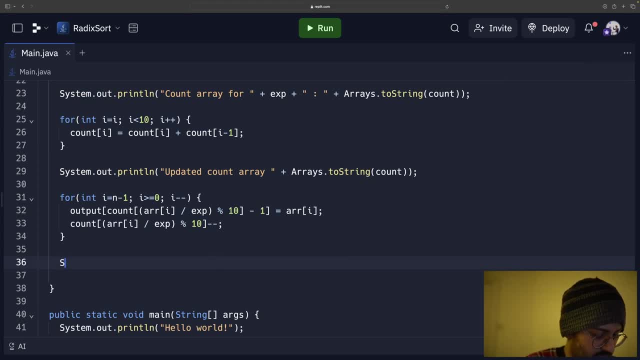 output with the main one. okay, and I will play it so you can see what what I mean. play it so you can see what what I mean. play it so you can see what what I mean. just give me a second system dot array. just give me a second system dot array. 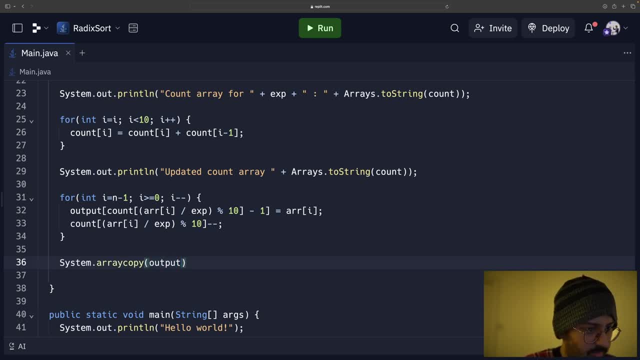 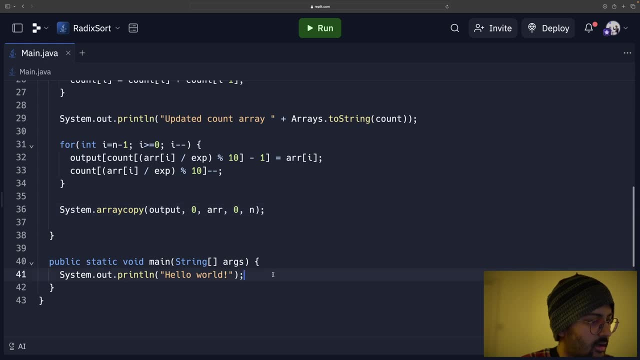 just give me a second system: dot array: copy out, put from the 0th in array 0 till. copy out put from the 0th in array 0 till n. Let me just run this So: 2983, and I will show you why I did these two things. 2983,. 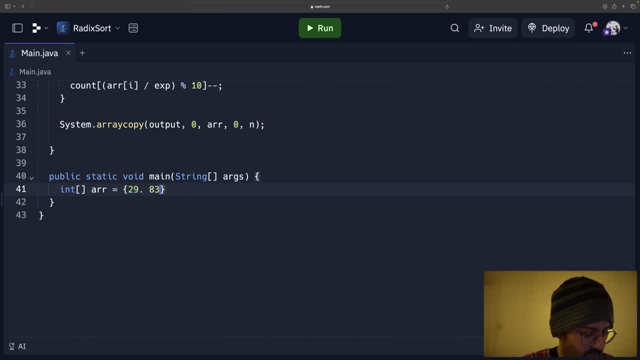 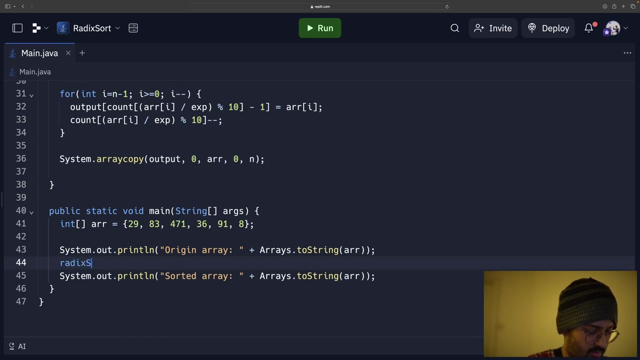 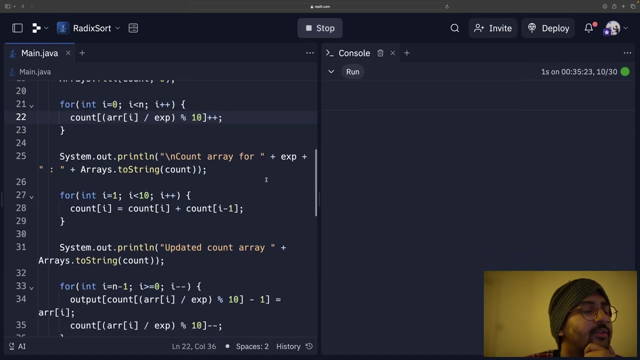 471, 2983, 471, 36918,. systemoutprintln origin: additional array: sorted array: arrays.2stringarr, and I will just say radix, sort, arr. Let's run this and now you will be able to understand. Okay, so if I run this, you will see what. 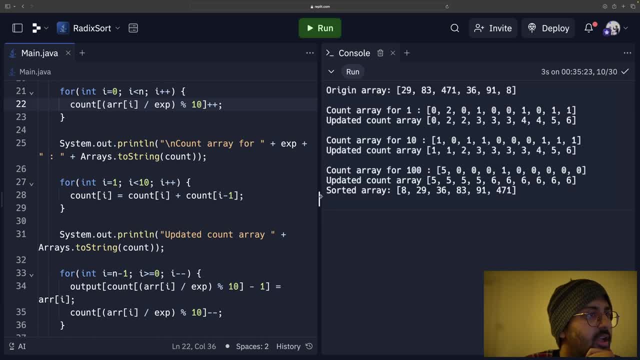 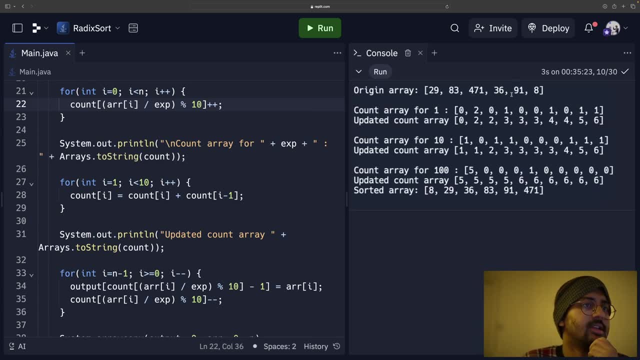 I mean, Here we go. So here I can see that, let's say, original array is this: Count array for 1 means base number 1.. So 9 is coming once, 8 is coming once. So 9,, 8,, 7 is not coming. 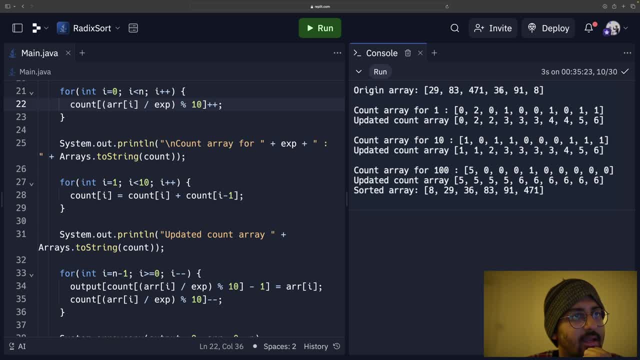 6 is coming once here, 5, no 4, no 3 once 2, no times. 1 is coming twice, like this. Okay, and then I did an updated count array, So for every index I added the previous index. So 2 became 2, this 0 became 2, because 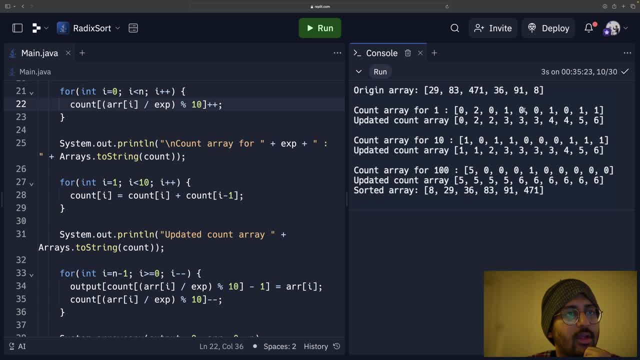 0 plus 2, 2.. 1 became 3.. Okay, this index also became 3, because 0 plus 3, then 0 plus 3, 3.. 1 plus 3, 3.. 1 plus 3, 4, 0 plus 4 plus 0 plus 4, 4, 1 plus 4, 5, 1 plus 5, 6.. The reason I did: 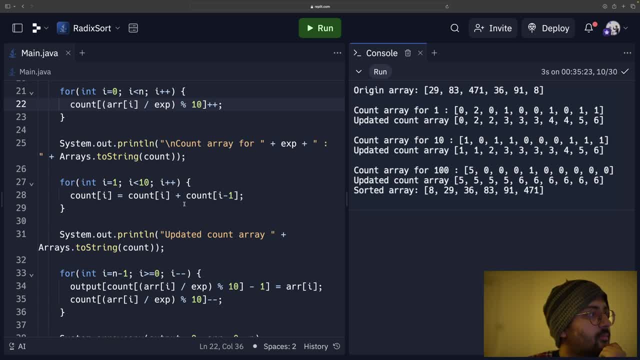 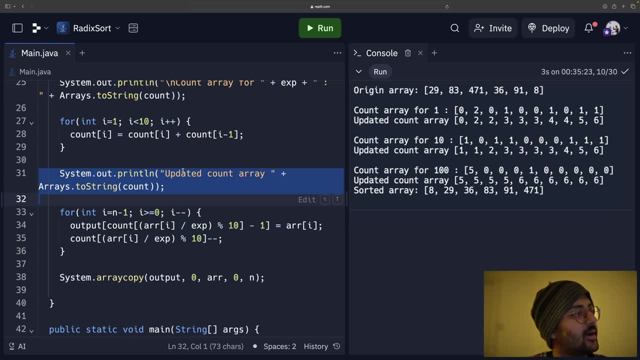 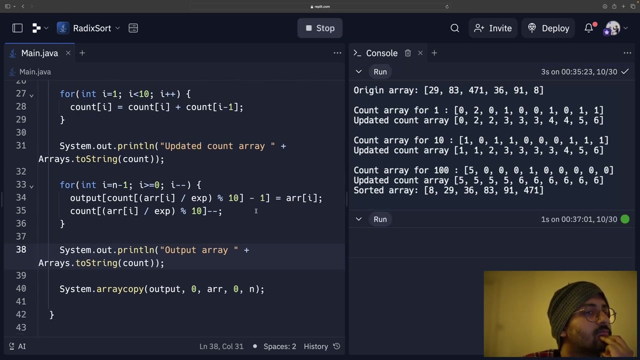 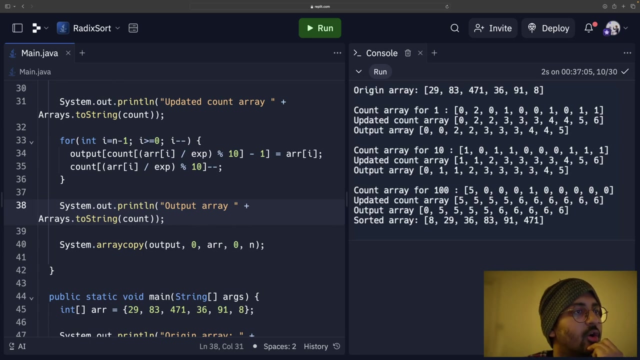 that is actually I updated count array. I should show you updated. I should show you the output array also The output array, Output array. See, now you're seeing output array. So for output array, it's saying that start from the last element. 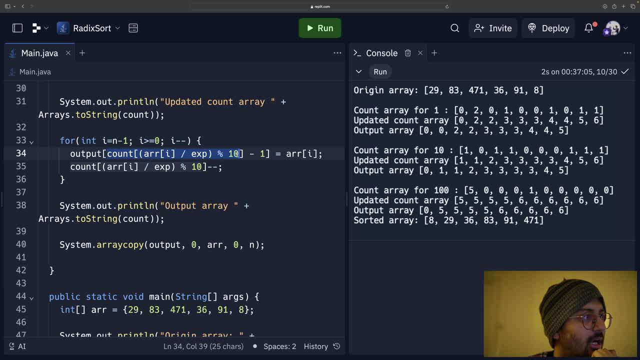 So output of this index right minus 1 is equal to arr of i, because I know that the arr of i is the main array, so the index in that array. okay, if I'm saying that the- let's say the element is, let's say, 91, okay, at index number one I have 91, not at index number one. 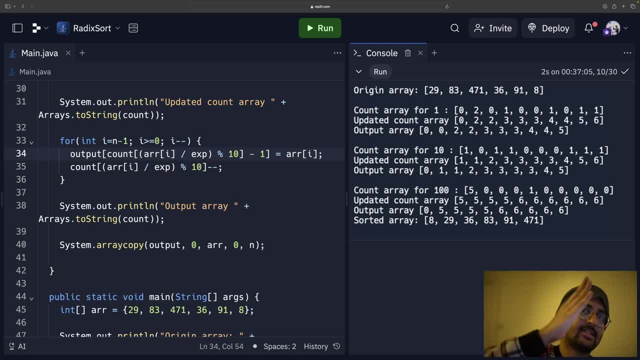 but you get what I mean, like, because I'm talking about the places. so let's say: first loop is first place, ones tens hundred thousand. so if I'm at the ones place, I'm saying that you know I'm starting from the very last. so output array: very last it's going to write output of, it's going to say the. 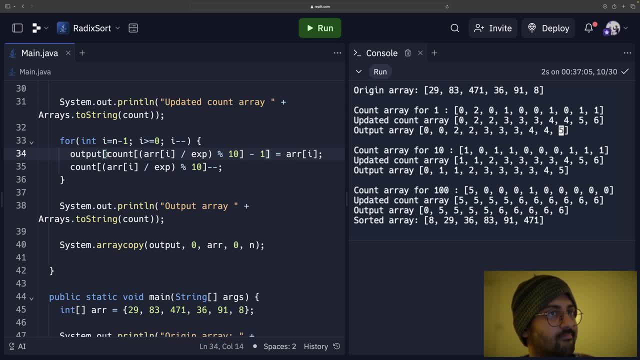 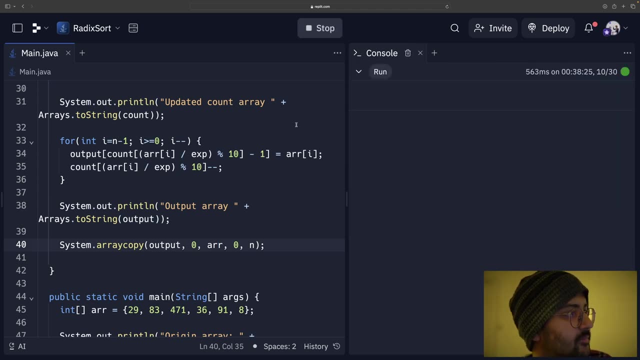 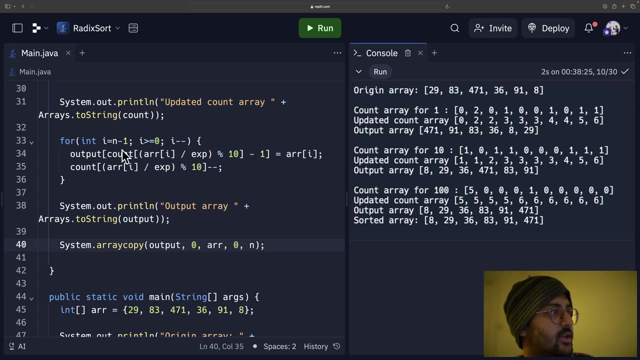 you know? oh no, it's printing count. I have to print output. that's why it was confusing. hold on. now you can see it is sorted based on the index number one. so here I'm saying at the last element. so the last element is actually equal to arr of ie. so 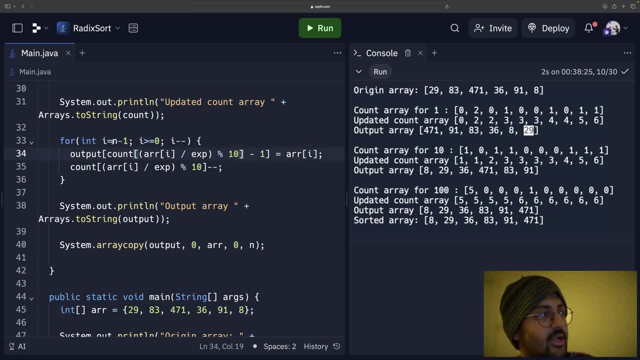 arr of not the last element, sorry, the last element of the original array. so the last element of the original array, which is 8, will go where 8 will go wherever the value of 8 is in my count array, Because I'm sorting it based on 8, so I will see where the value I have 8 for in my count array. 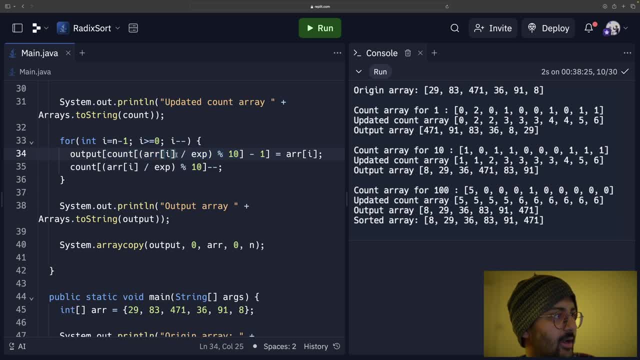 So count of a r out of i, which is, let's say, 8,, 8,, 8, minus 1, 7, because the value of 8 will be at 7.. So 0, 1,, 2,, 3,, 4,, 5,, 6,, 7.. So here in the output array, at 0, 1,. 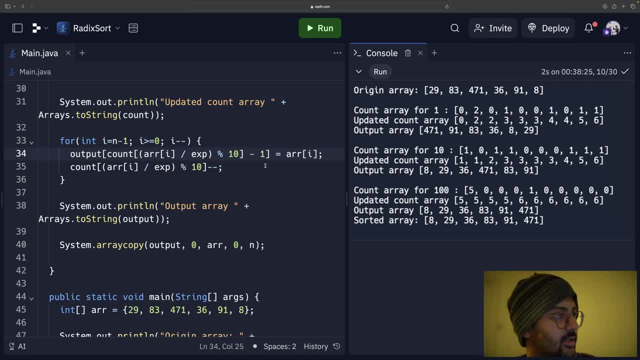 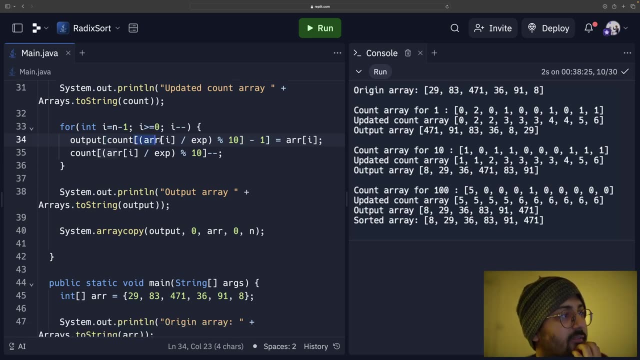 2,, 3,. no, not 7,. count of the a r out of i, which is giving me 8, minus 1.. So this is what I mean. Count of this thing is what Count of 8.. So 0,, 1,, 2,, 3,, 4, 5,. 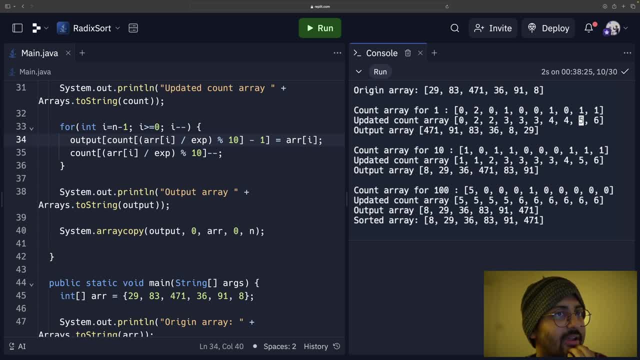 6, 7, 8, which is here at index number 5, minus 1, 4.. Here is actually going to have 8 over here, So here we have 8.. So here is actually going to have 8 over here, So here we have 8.. So here we have. 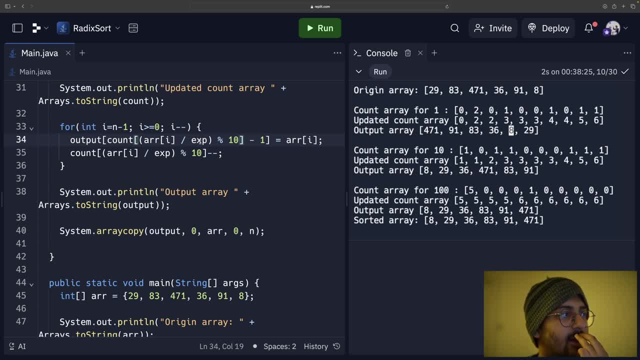 count of AR out of IE divided by 1, 8.. So, at 8,, what is count of 8?? Count of 8 is 0, 1,, 2,, 3,, 4,, 5,, 6,, 7,, 8, 5.. No, because we have added it ahead. So here I have 6. 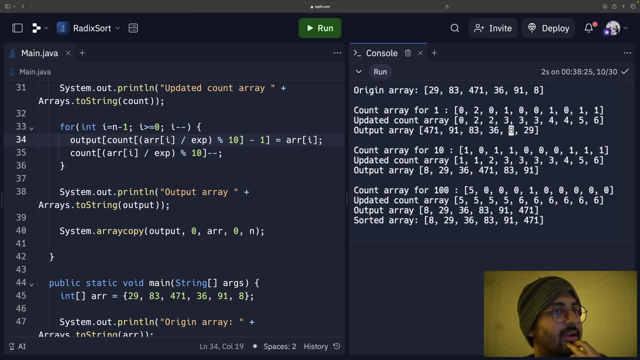 and 6 minus 1 is equal to 5.. So at 5 index I will put 8.. Similarly, when I run for this code- let's say I have the updated count array- like this, because I want to make sure that: 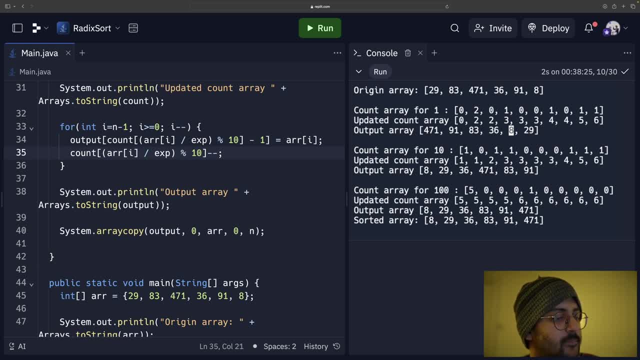 count of I. here in the updated, I want to say count of I- contains the actual position of this digit in my output array. Actual position of the digit in the output array. Okay, I can say if I'm over here again starting from n, yeah, you get the idea. I'm starting from this. now the array is this: 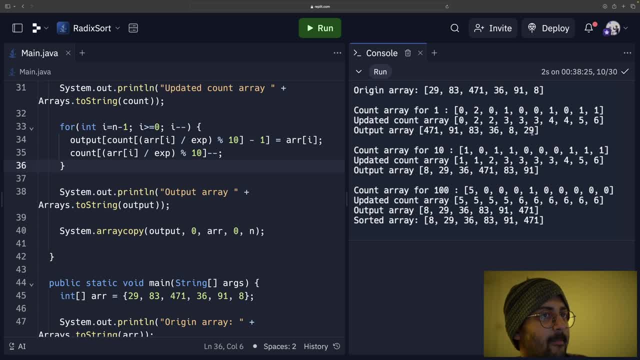 So I'm starting for 29.. I can say that output of count of- I can say AR- out of IE divided by 10, 2.. I will get 2.. Count of 2 is here. I am getting 2 minus 1, 1.. So 29 will be at index number 1.. Yeah, that is correct. 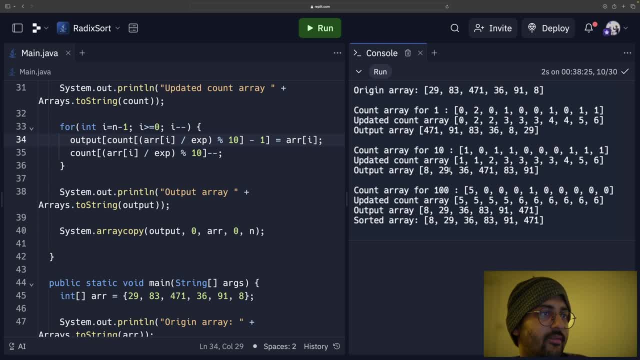 Index number 1.. That is how it's looping for every single. So this is for 1's place, 10's place, 100's place. Okay, I'm just mapping it. You can see it's just mapping. First I created the count array. 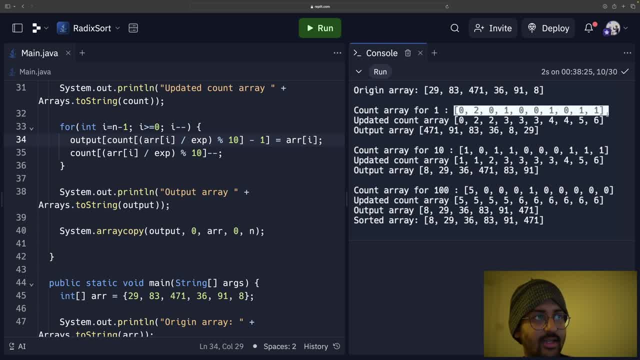 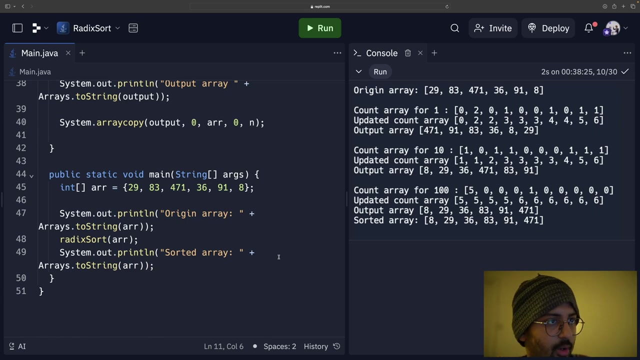 the frequency array. Okay, this is the frequency array. Then I updated the count array so that it represents the actual position of this digit in the output array. Okay, Cool, Sounds good. I'd recommend, if you're confused then try to dry run it, Use the debug pointer. 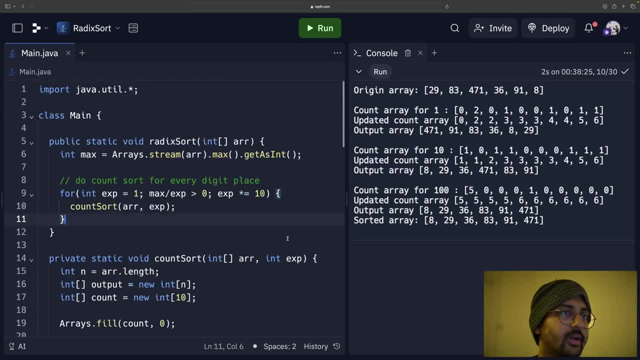 and run it again. It will be straightforward. But yeah, if you have any questions, let me know in the comment section below, And that's pretty much about it. One thing I have to tell you is the time complexity. So total times the loop is running outside is the digit. 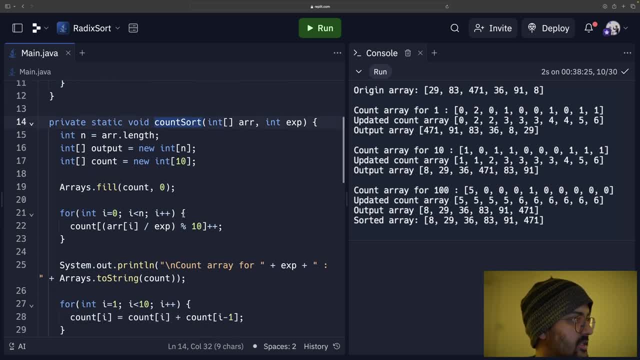 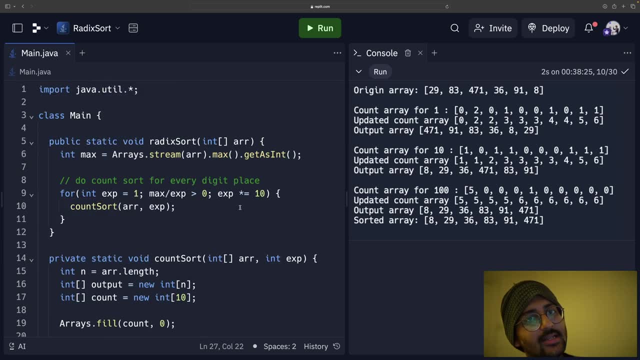 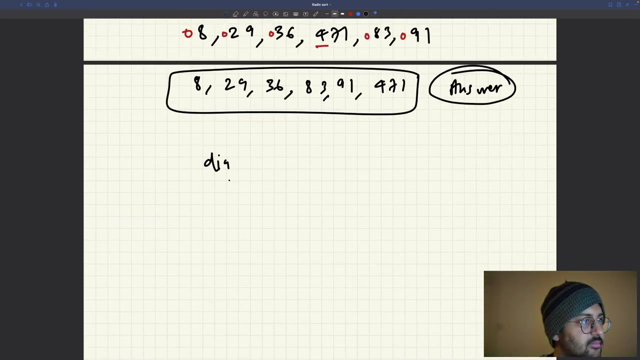 So digit multiplied by what is the complexity of this? N plus 10.. So base, whatever the base is, So time complexity is digits multiplied by, or I'll just write it here: Okay, Digits multiplied by N plus base. Okay, Sounds good. So when I talk about radix, sort that's, 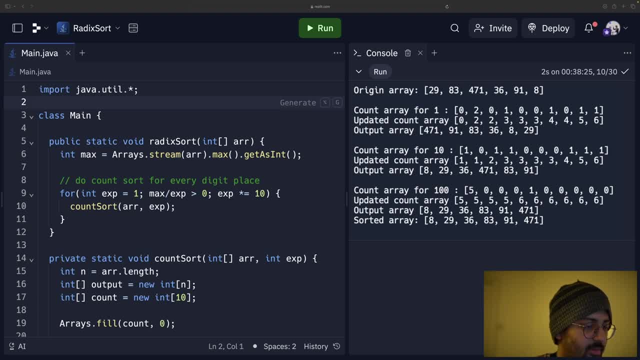 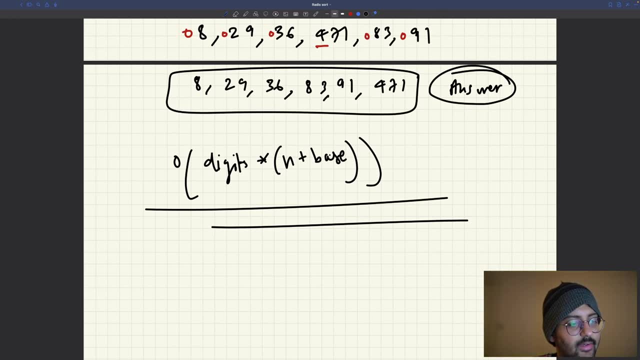 the time complexity And, as you can see from the time complexity, well, we are using an extra space as well over here for count arrays. Okay, So let's talk about the time complexity. So it is like you know faster as compared. 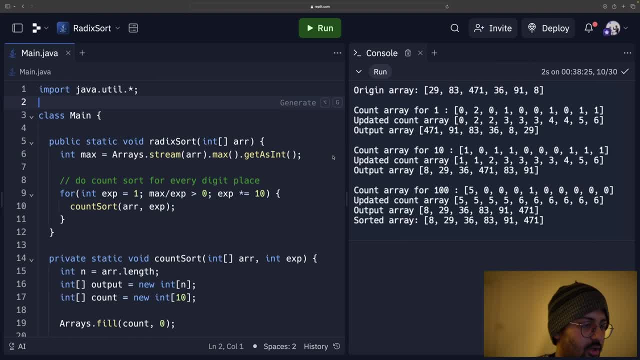 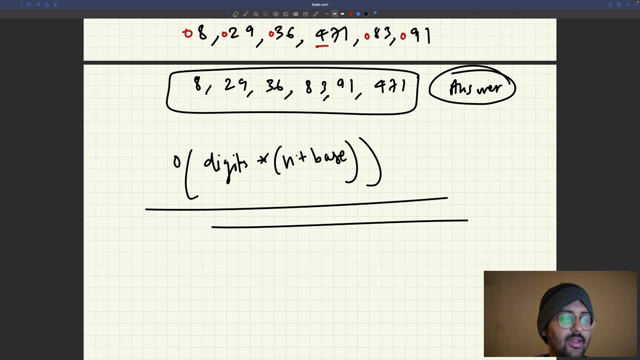 to other comparison based sorting algorithms like quick sort, merge sort, When you talk about large databases. but you can see, since it depends on it's growing linearly with the number of digits, So it's not very efficient when we talk about smaller numbers. okay. 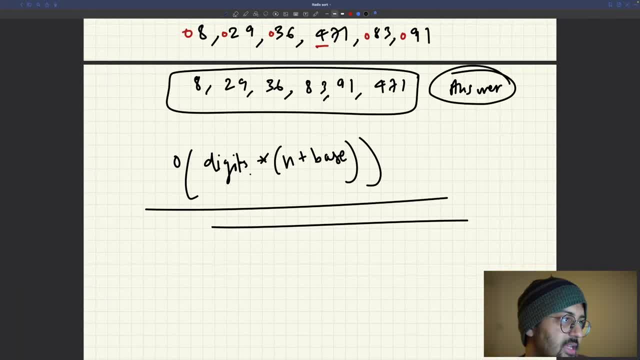 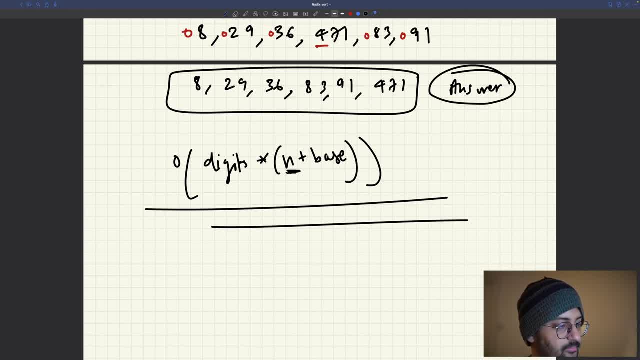 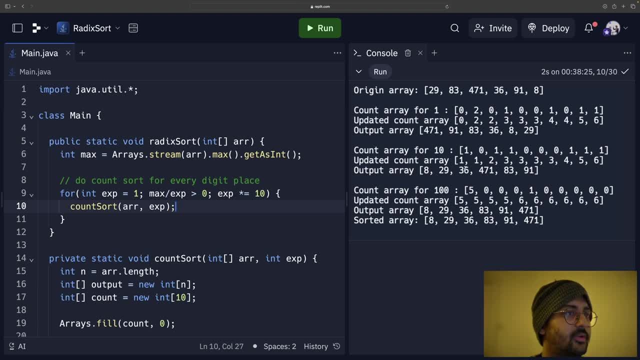 grow right. so, yeah, cool, try to dry run this. see in pen and paper if you, if you write it on pen and paper, every single step for updated count array, you will understand, okay, what we are doing. but the whole idea was trying to get then the where this lies in the output array, the digit. okay, as I showed you in the 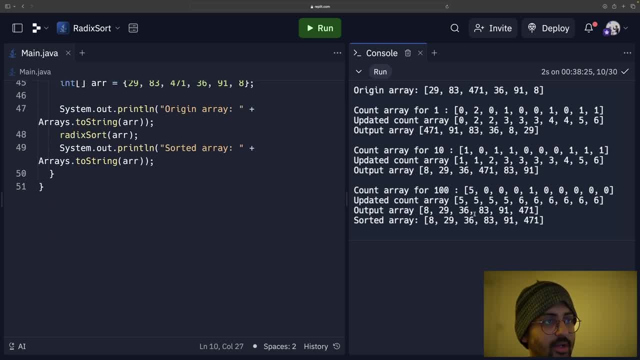 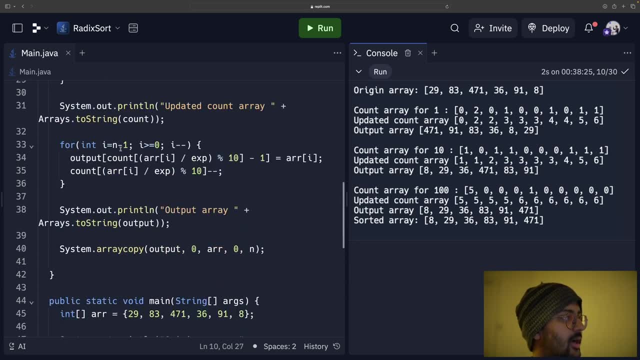 examples. I can take another example. let's say this is the output array, this one, okay, and I'm talking about. let's say I go back over here I say, for I is equal to last index, or that's it. I is equal to second last. let's say 80, second last.